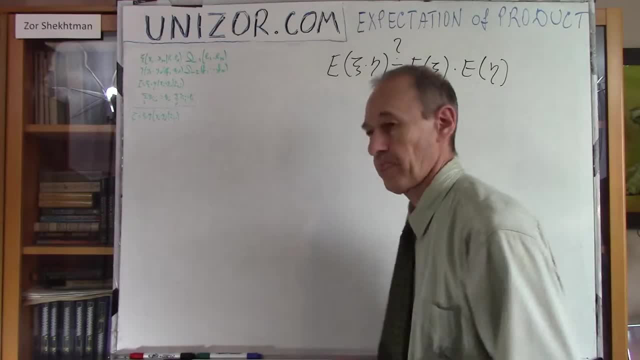 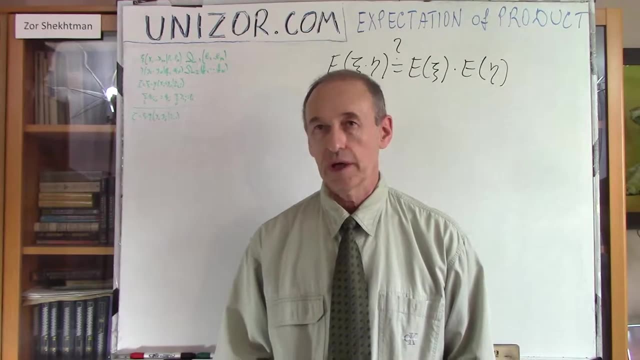 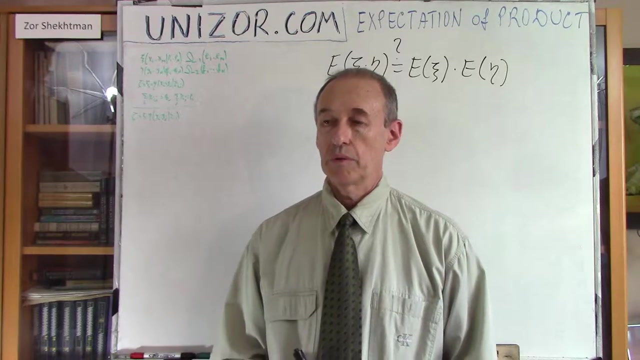 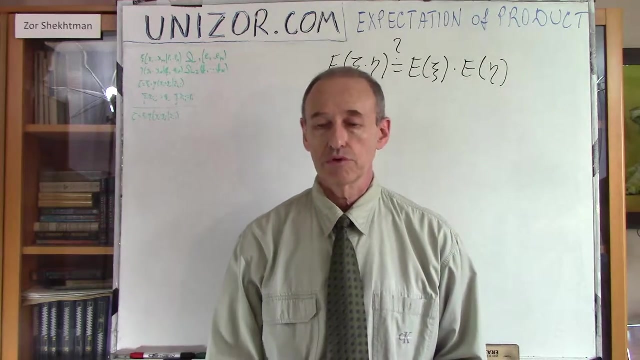 Hi, I'm Zor. Welcome to UniZor education. I would like to talk today about mathematical expectation of the product of two random variables. While this lecture is part of the course of advanced mathematics presented on uniZorcom, I recommend you to watch this lecture from: 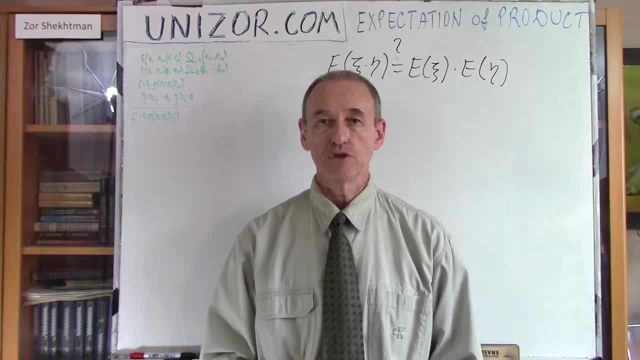 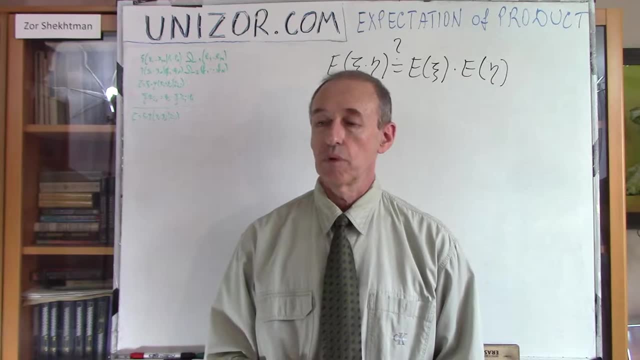 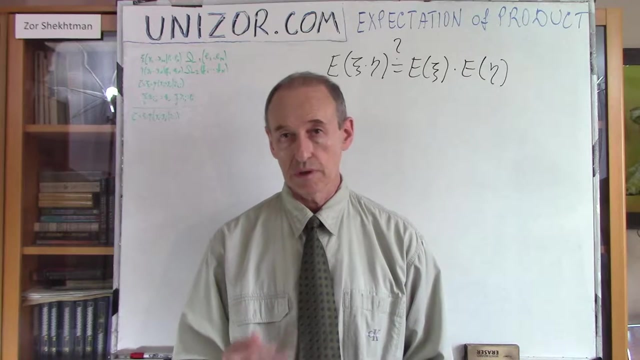 this website because it has notes. basically the same information which I'm presenting as a lecture is in the notes, basically as a textbook. Well, besides, if you are on the website, there is certain educational process, the functionality which you can actually engage. 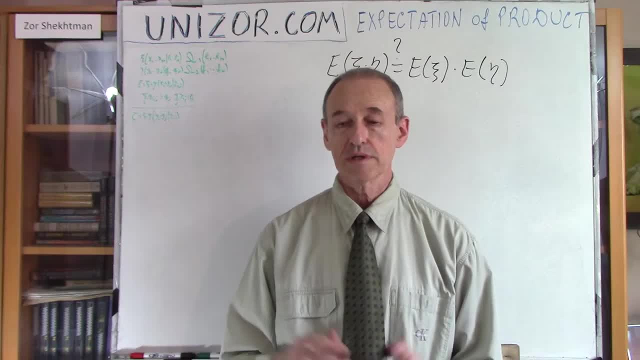 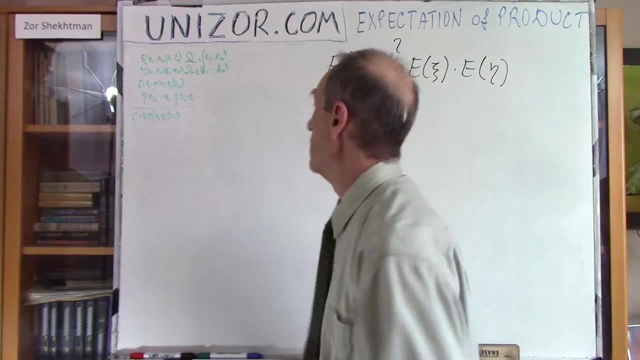 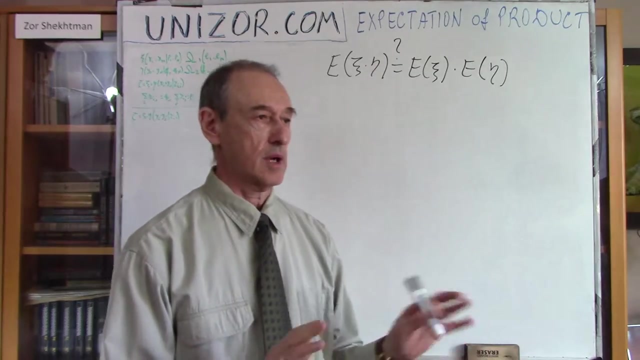 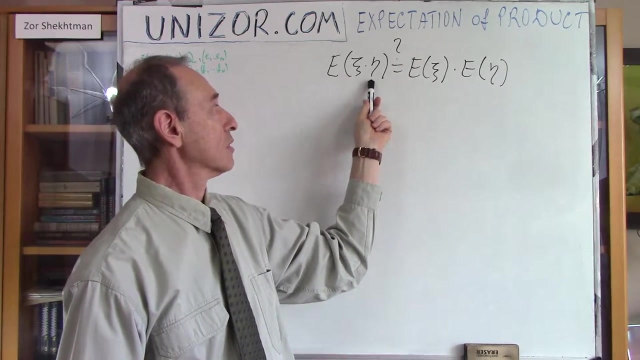 in which includes enrolling into the courses and taking exams, etc. And the site is free. So let's talk about mathematical expectation of the product of two random variables. Well, let me just upfront state something which we will discuss: Mathematical expectation of the product of two random variables is equal or not equal. that's a question mark. 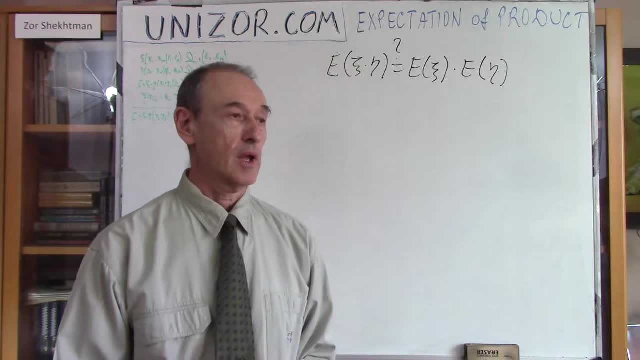 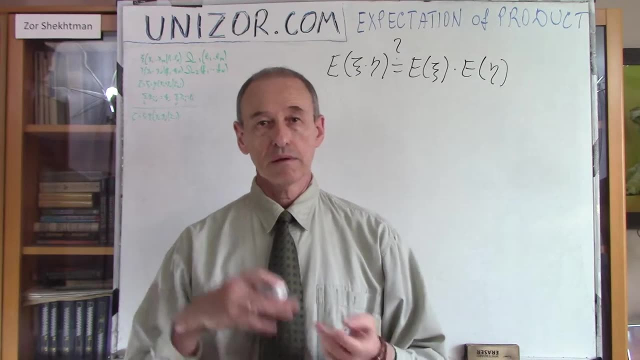 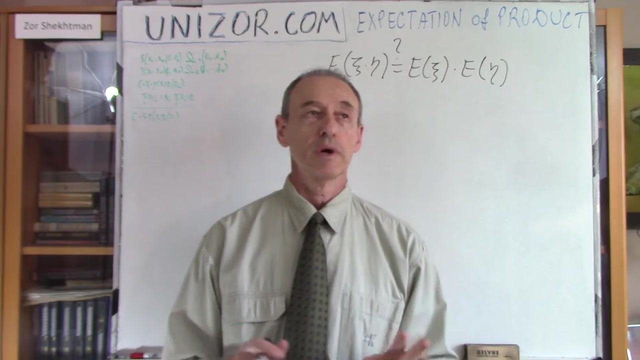 the product of their mathematical expectations. Well, first of all, let me just address this problem intuitively. We will not talk about mathematical expectation of the product of two random variables. It is quite analogous to mathematical expectation of the sum of two random variables. that I 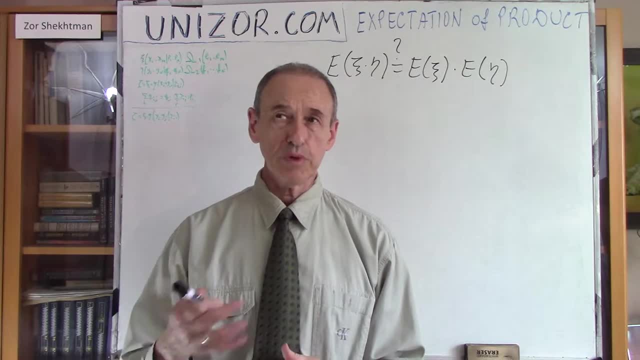 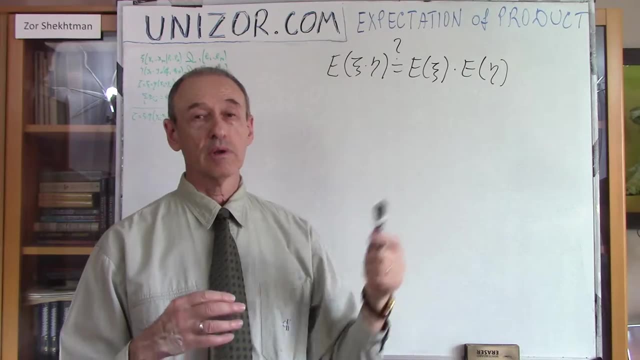 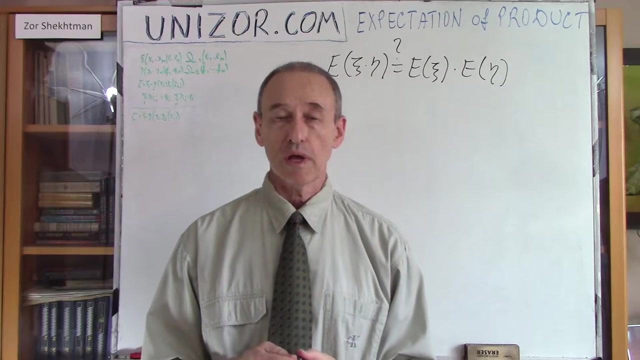 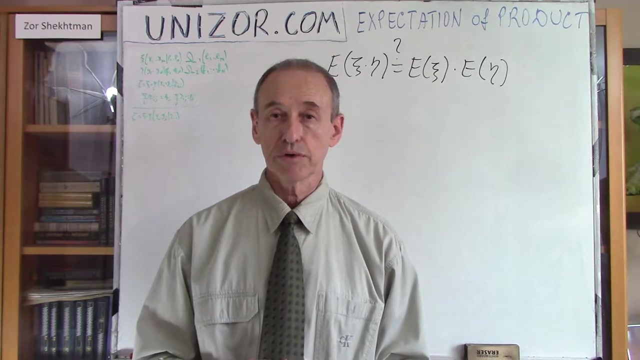 will talk about So intuitively. what is mathematical expectation? Well, people view it as a point around which all the values of the random variable are concentrated, So such and such. and then we measure temperature of 100 different people, and all of them are. 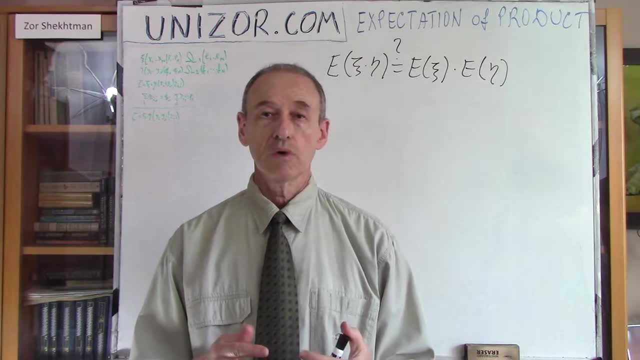 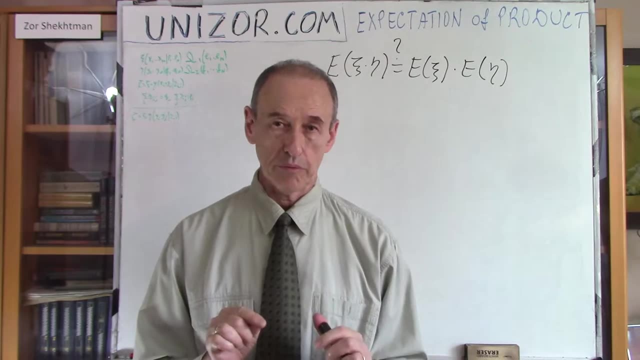 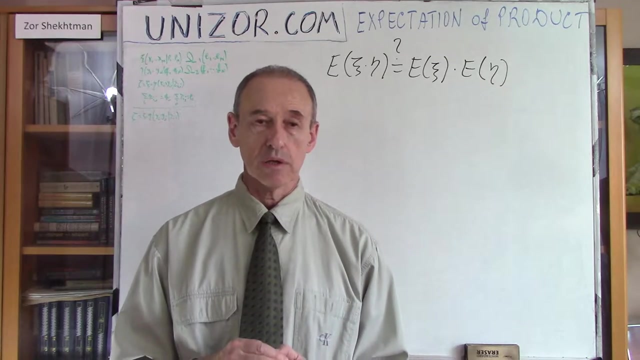 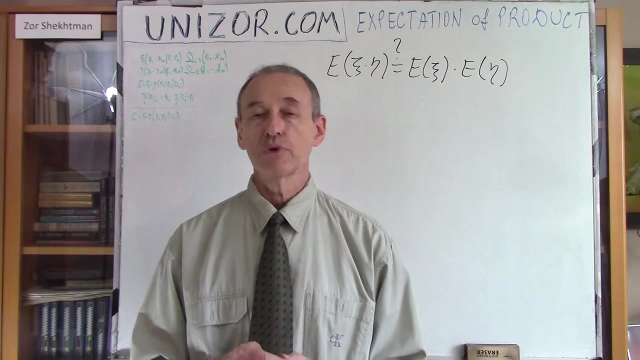 healthy individuals. their temperature will be different, obviously, but very much close to this so-called normal temperature, which is actually a mathematical expectation average, if you wish, of the temperature of a healthy body. Now, if you will take two different populations, let's say in, I don't know, United States. 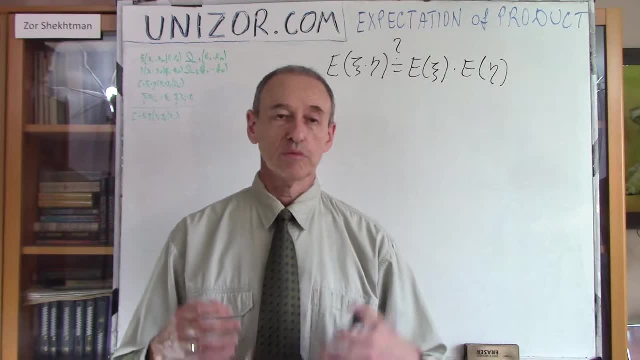 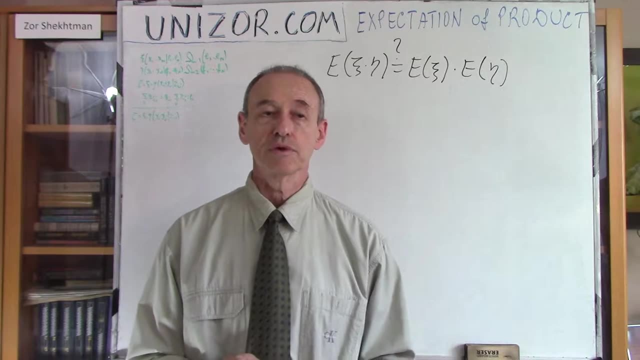 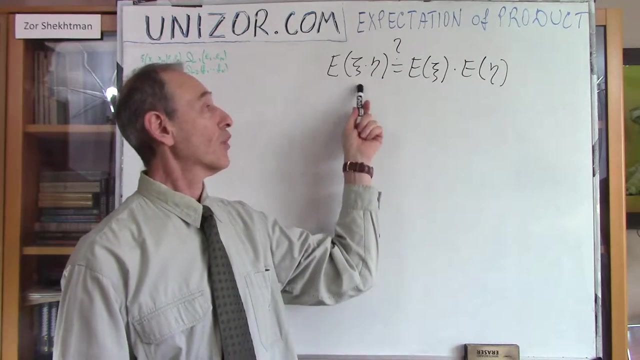 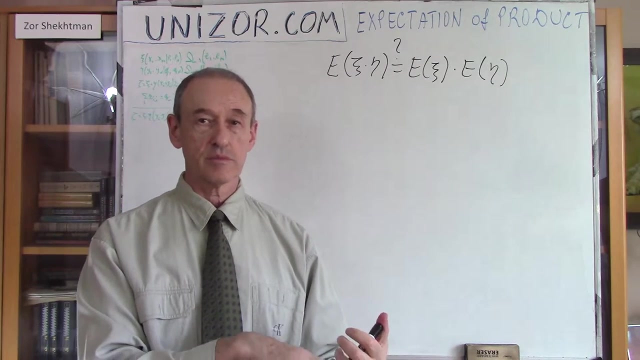 of America and China and you will measure the temperature here and there. well, they are kind of different right, Different group of people, but I'm pretty sure that mathematical expectation of the product of our temperature Temperatures- Temperature of one person from United States times temperature one person in China. 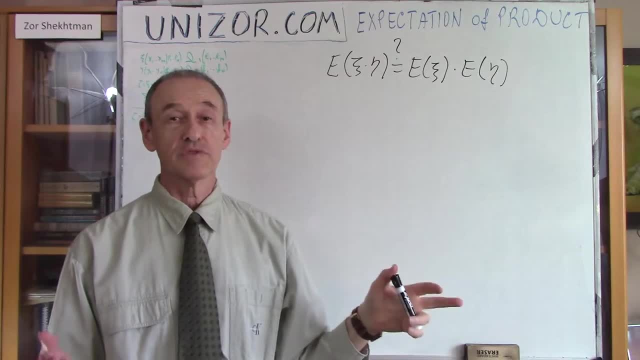 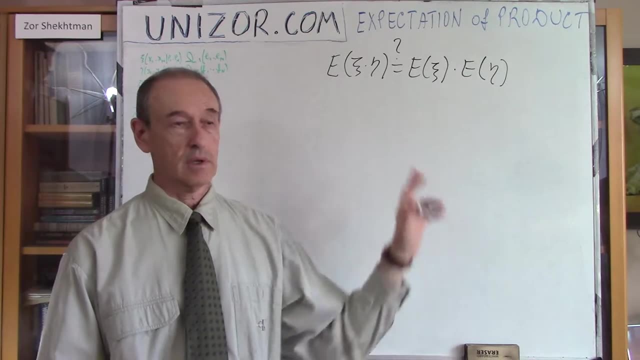 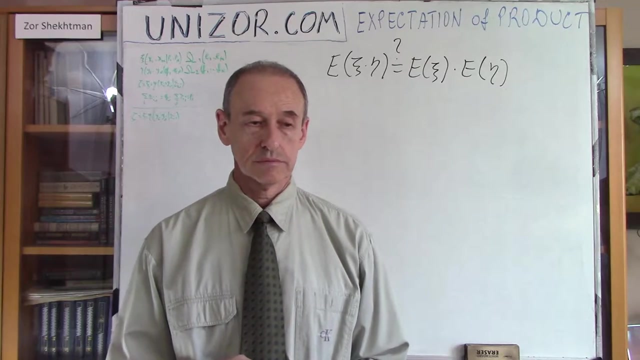 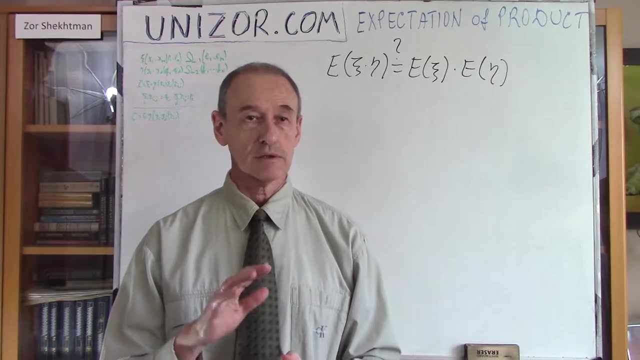 And we will take the mathematical expectation of these products. it will be the same as if we will just multiply separately the averages. So that's intuitive. Now I'm still thinking: Okay, Let's talk about this question mark. It's very, very important to understand that intuitive approach is not necessarily correct. 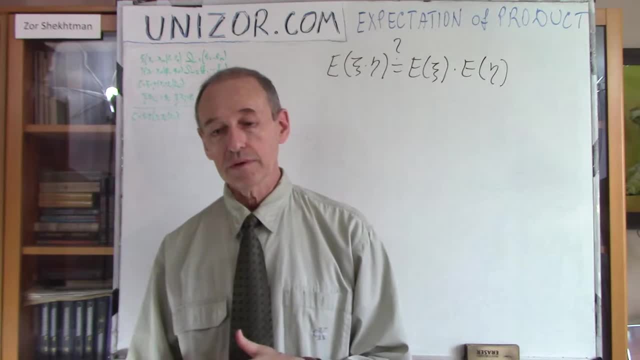 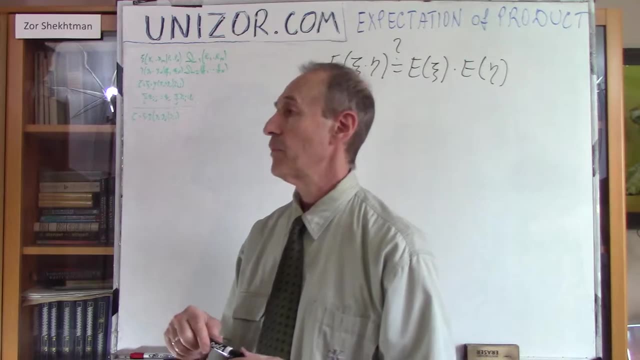 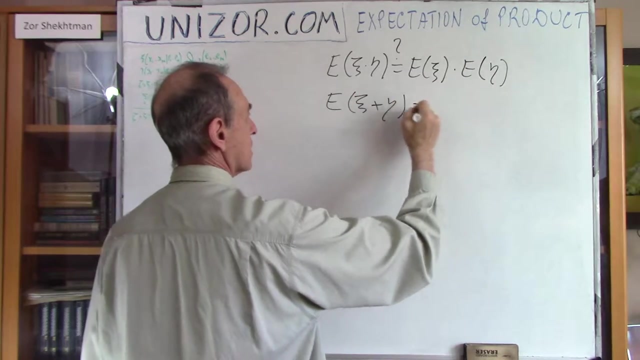 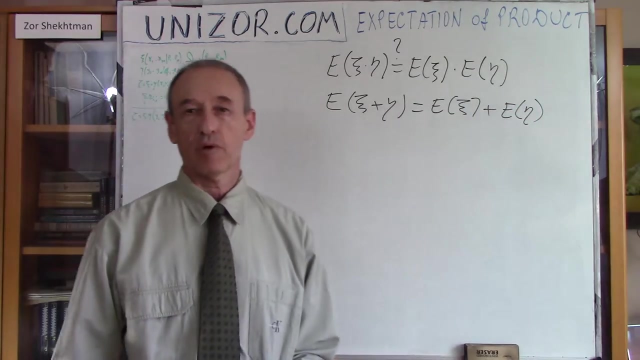 mathematically, But let's talk about sum of two variables, sum of two random variables. Now, with sum of two random variables, we have already proven that this is true. Okay, And what is this? In general, it is to prove something. 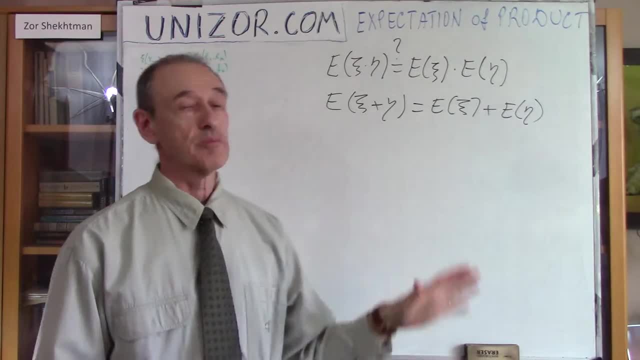 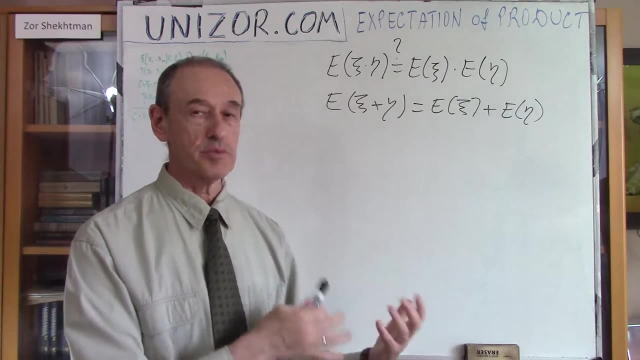 Well, indeed it is. The same thing can be proven for any pair of random variables, And let me just very, very briefly explain again. I mean, you can always refer to the lecture where it's proven, But I will just repeat this particular proof because I do need it for the product. 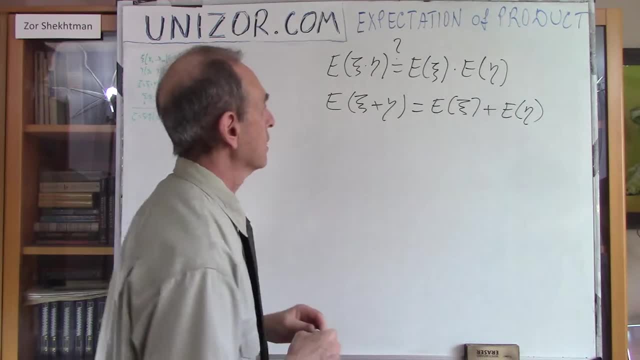 So how can we actually prove this thing? Well, let's imagine that we have two different examples, Never mind that we are only using one product. How can we prove that? Let's just say that we have two different mate of the same product. 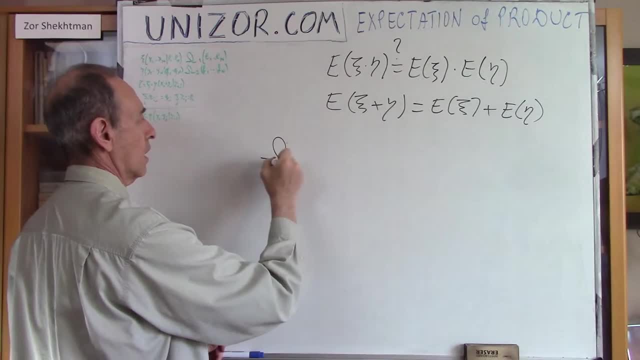 Why is that? Well, remember that I said that we use two types of variables because of the exact same result. So that's the basic thing we are trying to achieve, And our first answer is a different product. So let's just say that there are two different major variables. 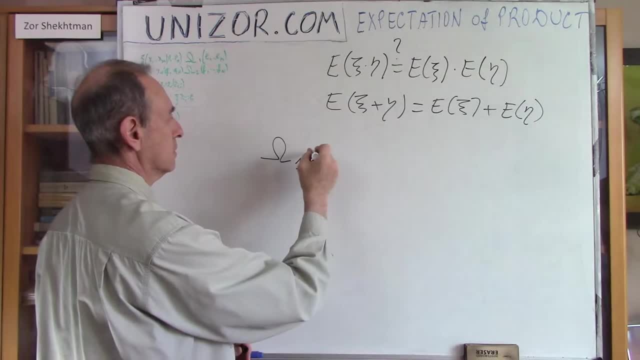 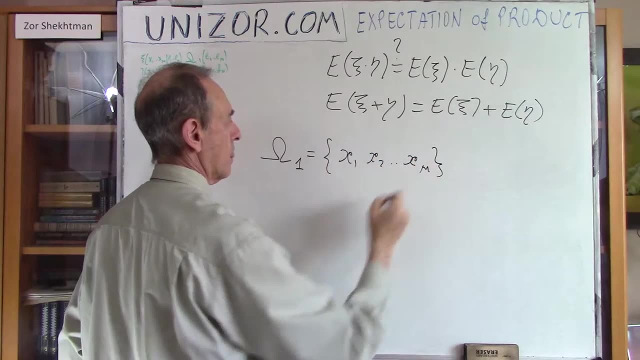 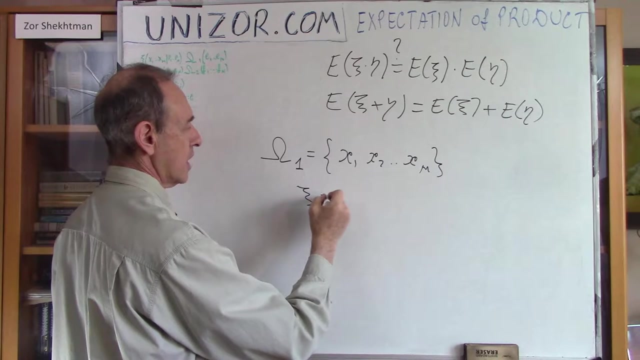 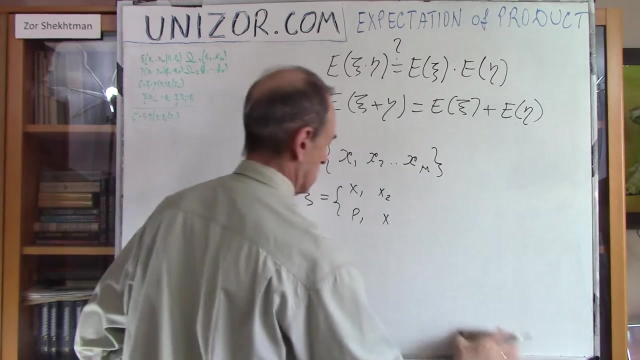 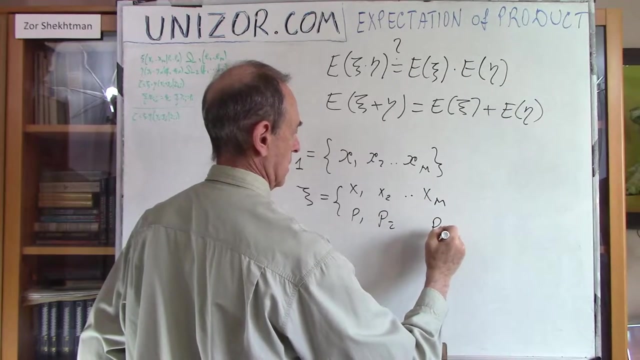 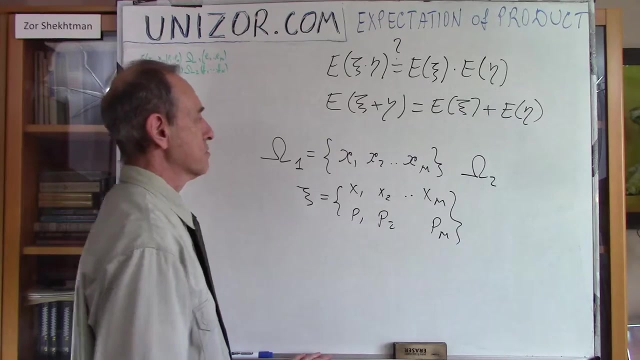 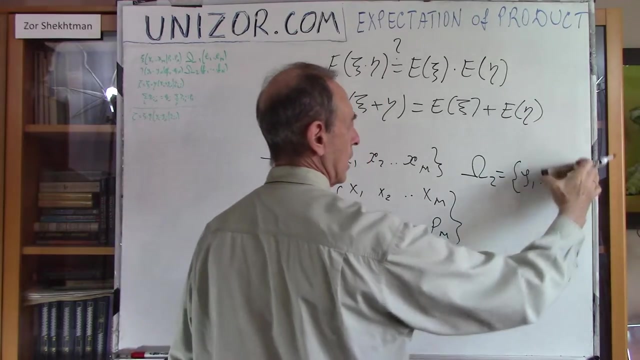 probability spaces q1,, which is values x1,, x2,, etc, xm, and we have the random variable xi, which takes these values with corresponding probabilities. And then we have another probability space which contains values y1, etc. yn- different number obviously, of elementary events, with 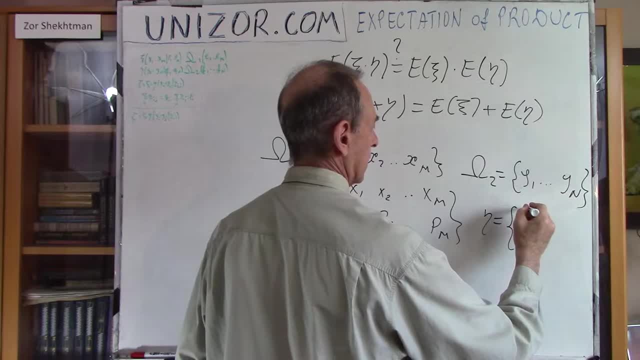 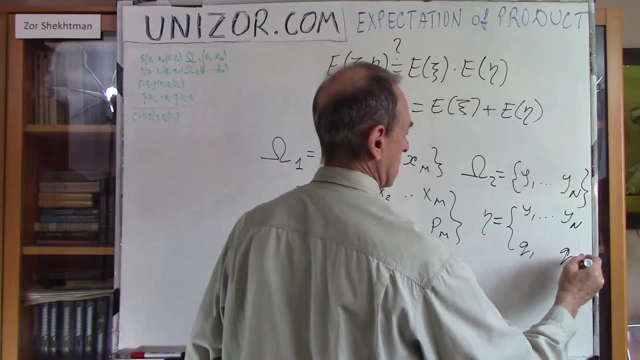 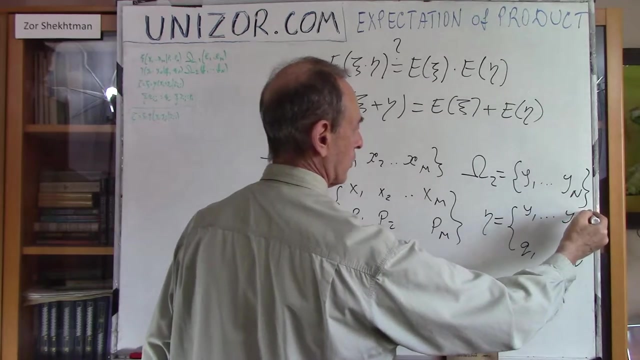 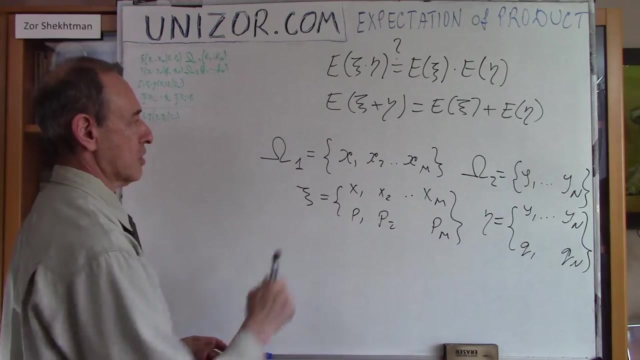 different measure allocated to each one: q1, qn. Obviously, sum of all p from 1 to n is equal to 1, and sum of all q from 1 to n is also equal to 1.. So we have these two random variables which are defined on these probabilistic spaces. 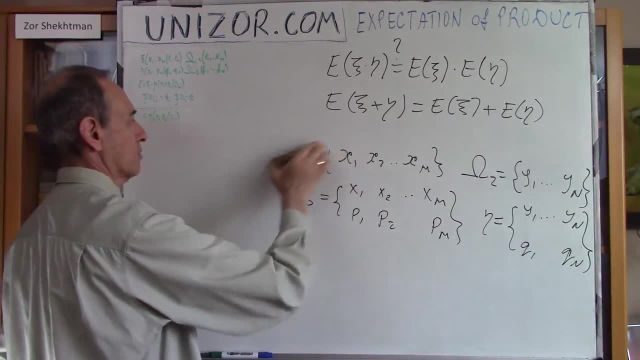 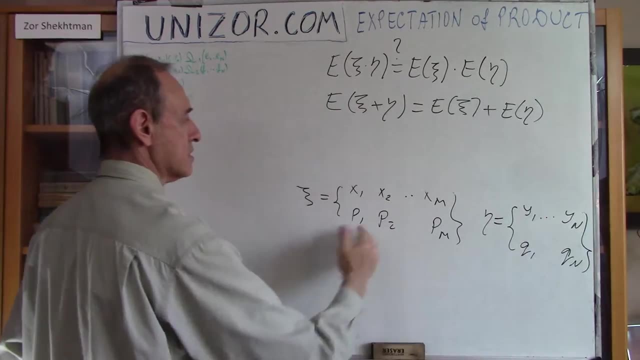 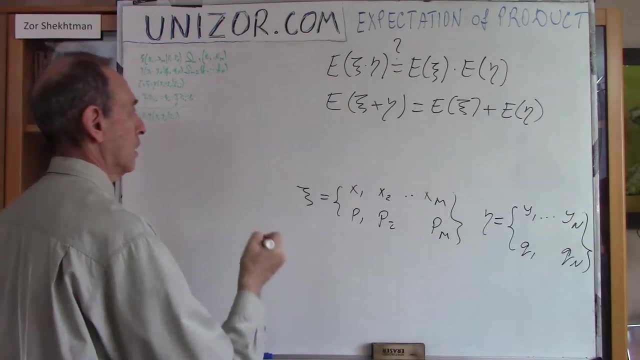 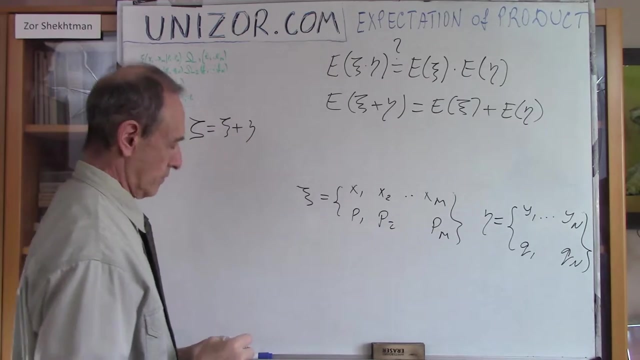 So basically, you can just say: forget about probability spaces. you can say that these random variables take these values with these probabilities. Now let's construct a new variable which is called xi plus zeta. Alright, The variable zeta. what values can it take? 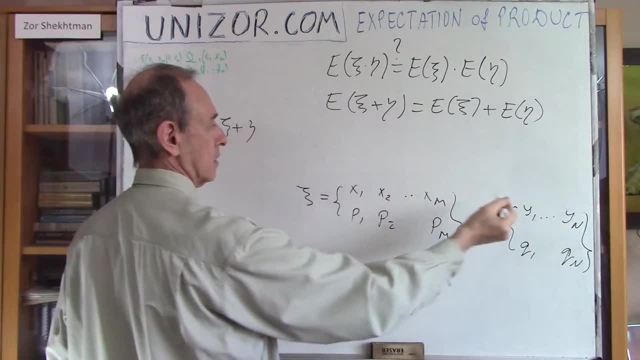 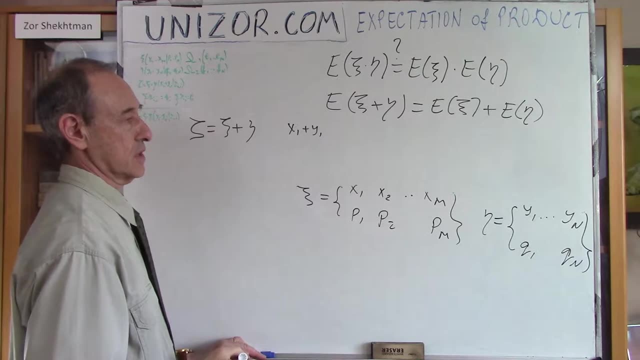 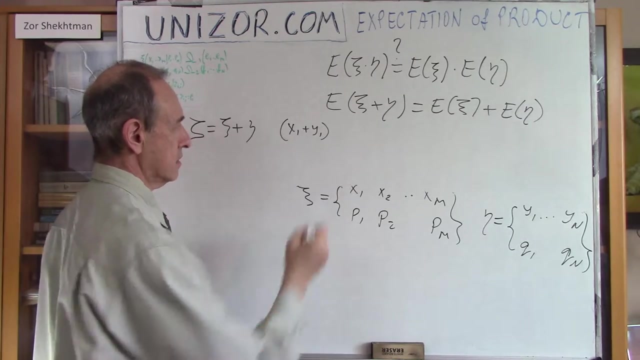 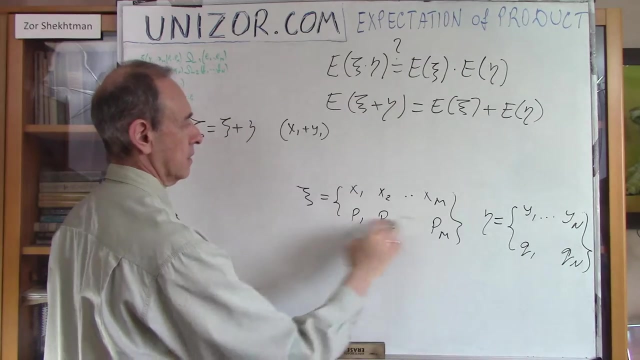 Well, it can take value, for instance, x1 plus y1, right? What will be the probability of this? Well, that's the probability of xi taking the value- the value x1, and probability of eta taking the value y1, right. 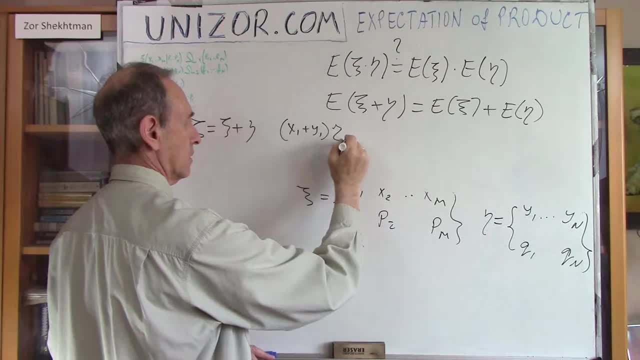 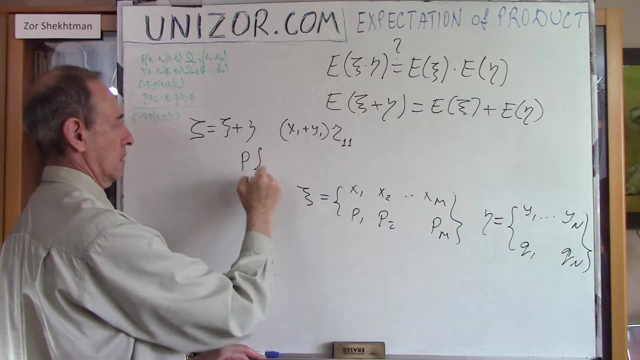 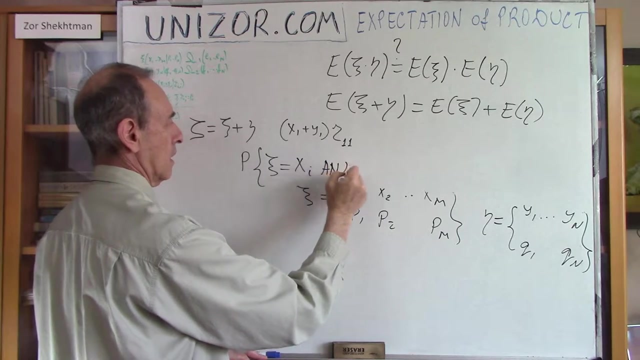 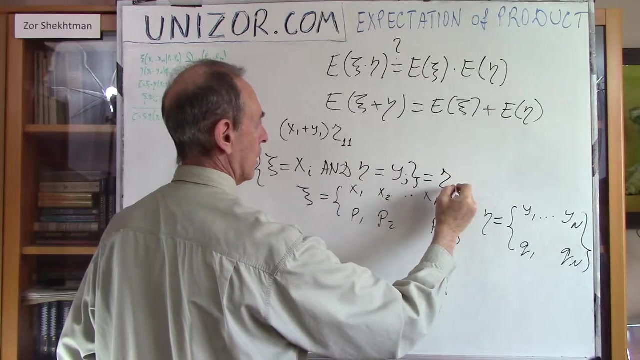 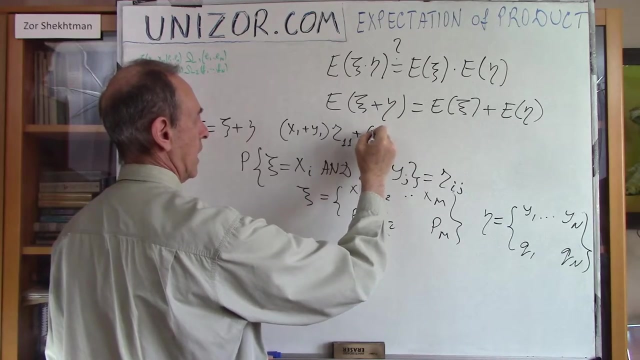 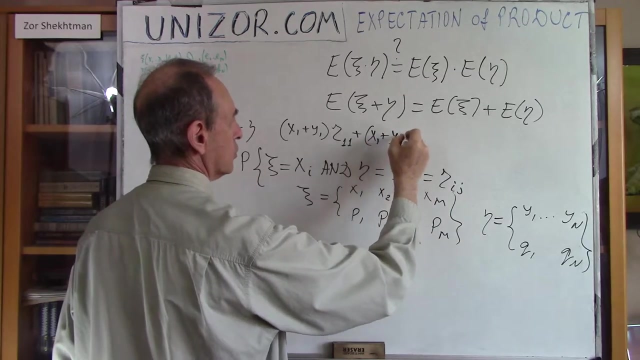 So let's call it r11.. So it's the probability of xi taking the value xi and eta taking the value yj, And this I call rij right. So plus Now my xi can take value x1, and eta can take value y2.. 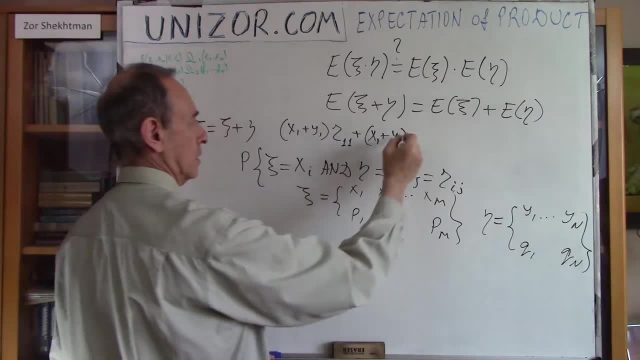 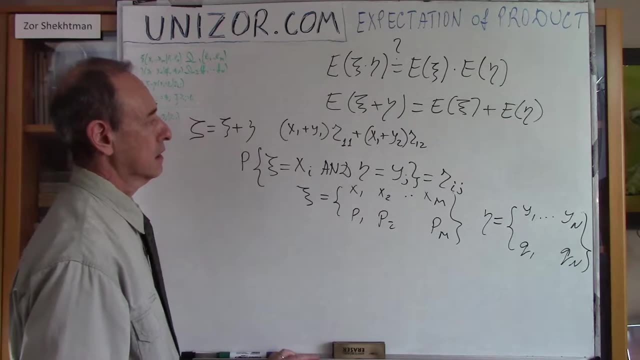 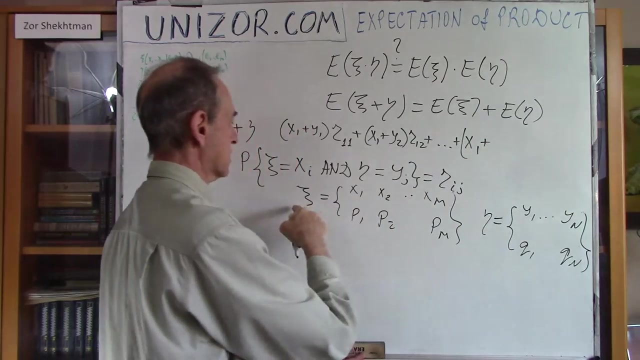 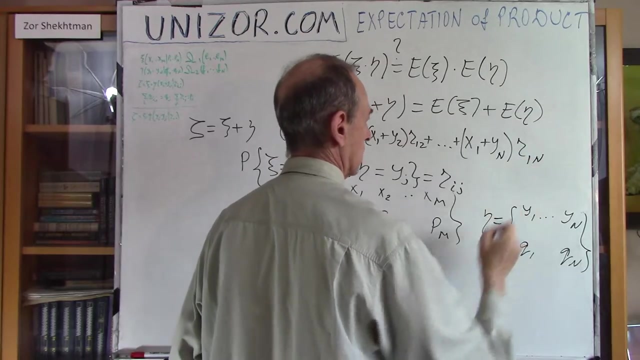 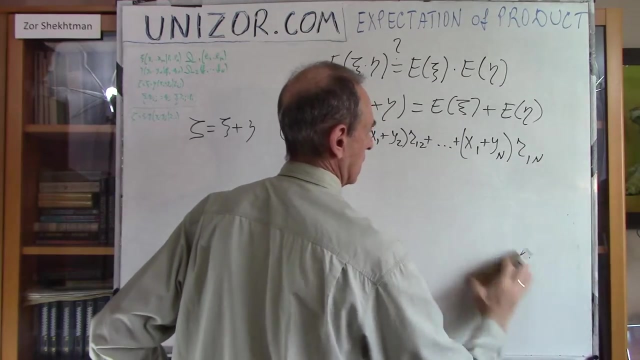 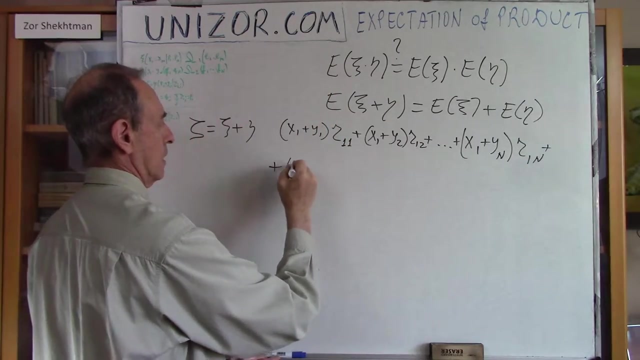 And what's the probability of this? Well, according to my notation, it's r12, etc. The last value with xi equal to x1, the value will be yn and r1n. Then my xi can take value x2,. 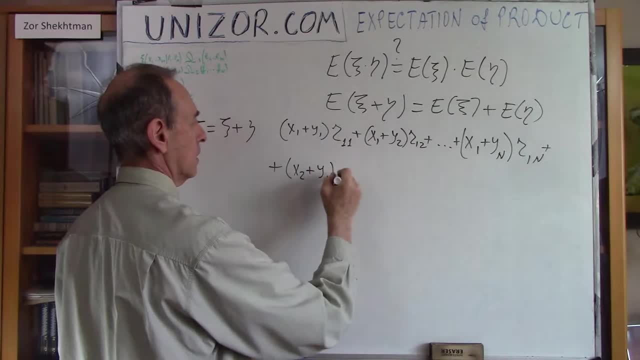 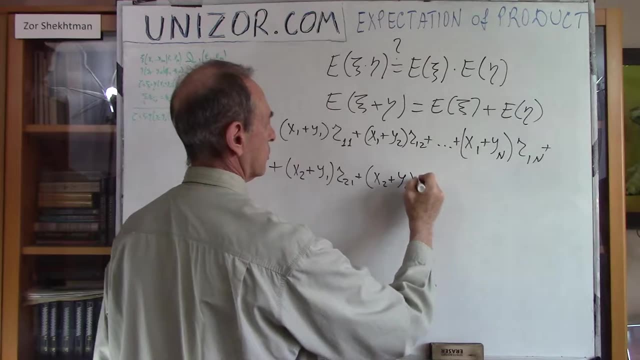 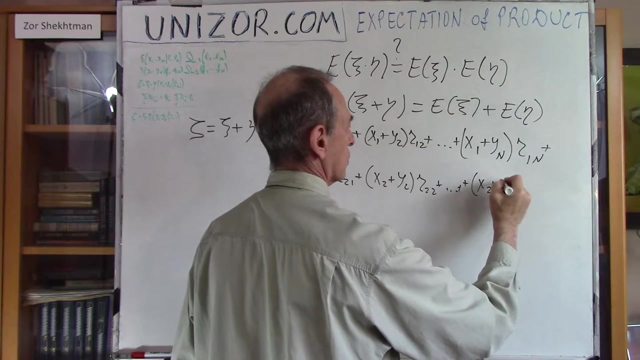 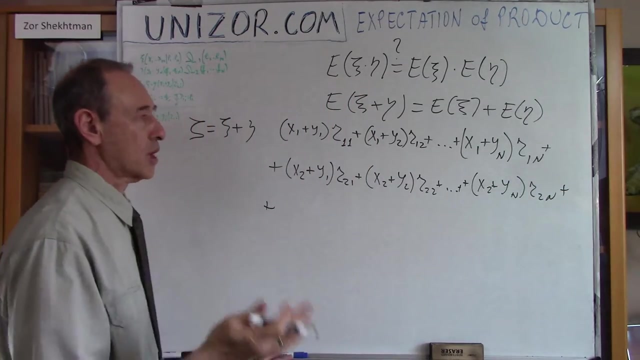 and eta can take value y1, and probability will be r21.. Also, x2, y2 would be r22.. And the last one in this row would be x2, yn. r2n+. So what are we doing right now? 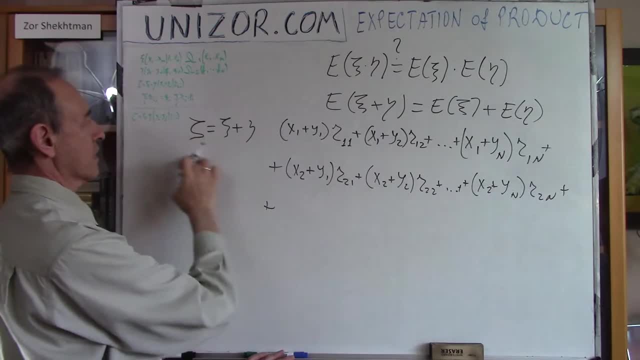 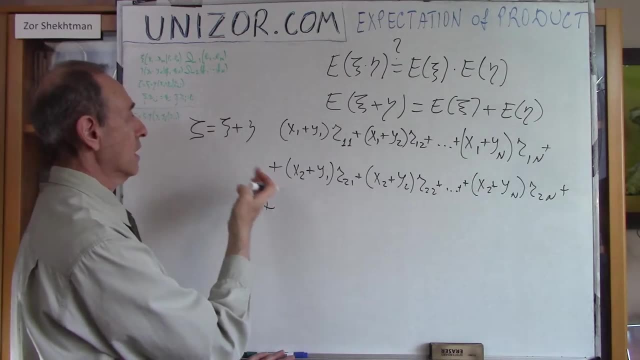 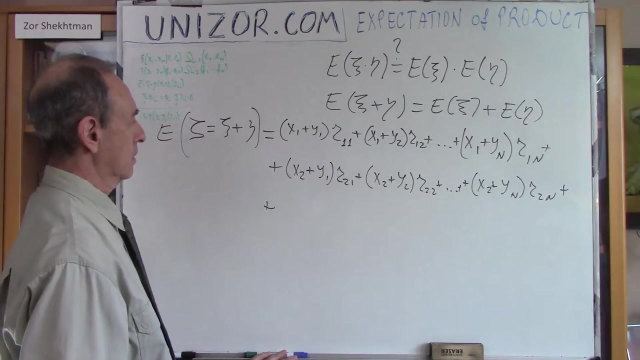 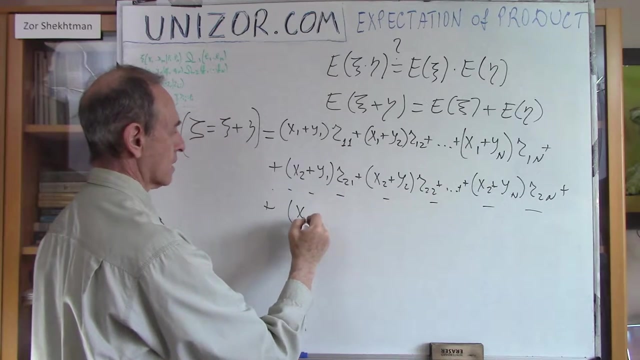 We are summarizing values of this variable times the probability of that value. So this is actually a mathematical expectation. That's what we are talking about right now. So, etc, etc, etc. It will be x3 plus whatever, and the last one will be xm plus y1,. 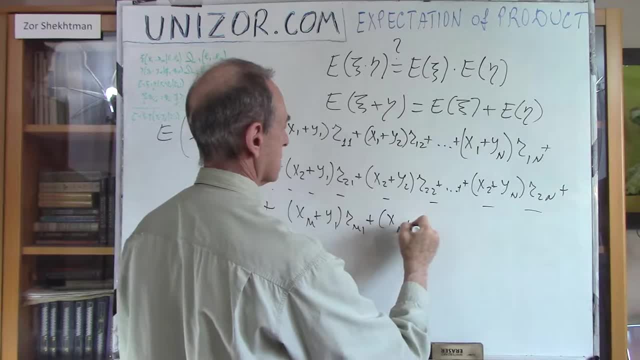 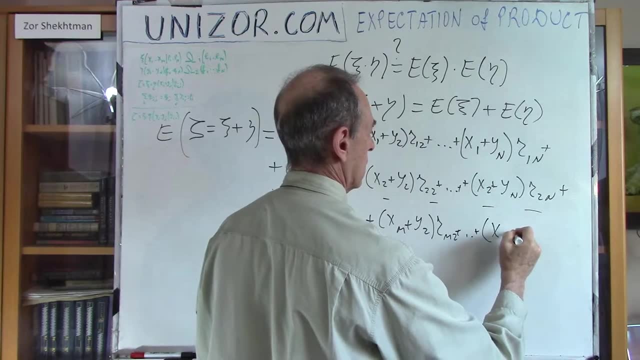 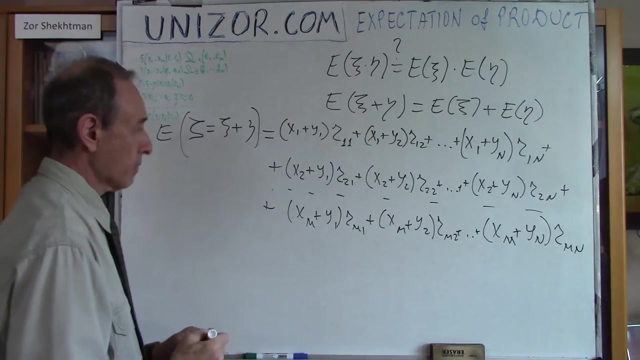 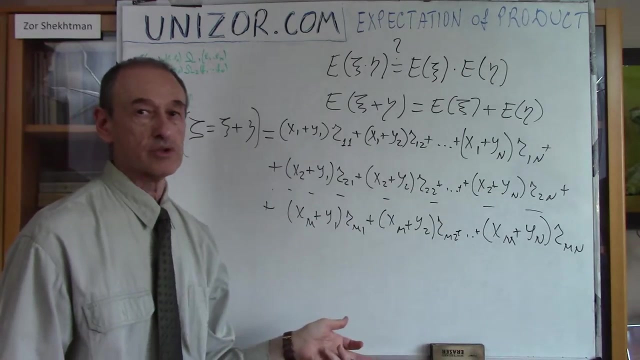 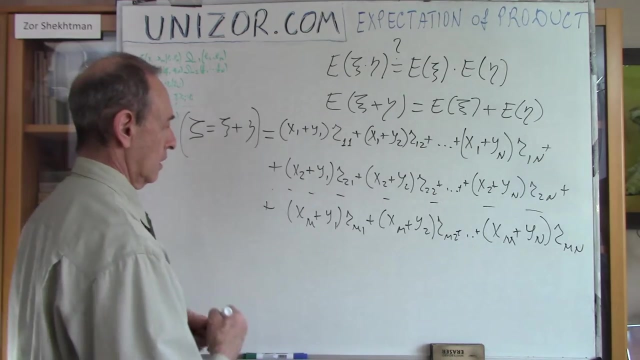 rm1 plus xm plus y2, rm2 plus etc. plus xmyn rmn. So that's my probability times value And we add them all together and that's how we form the expectation. But now let's regroup this. 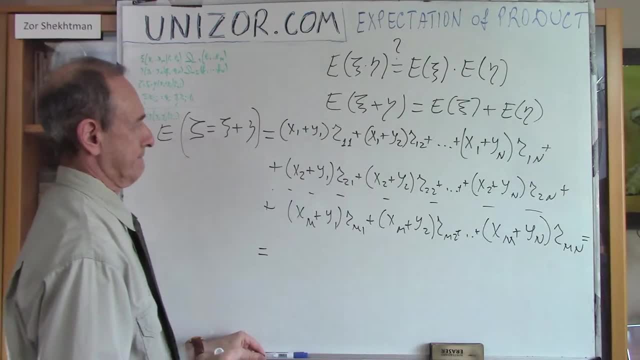 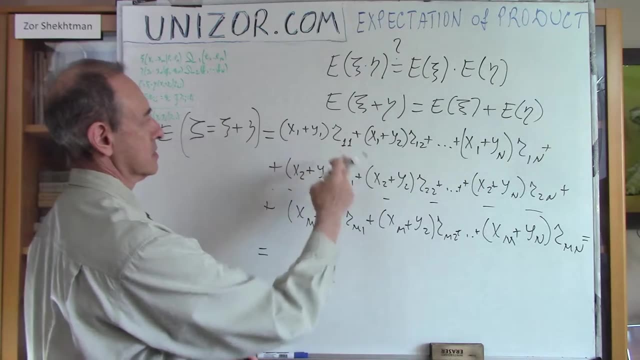 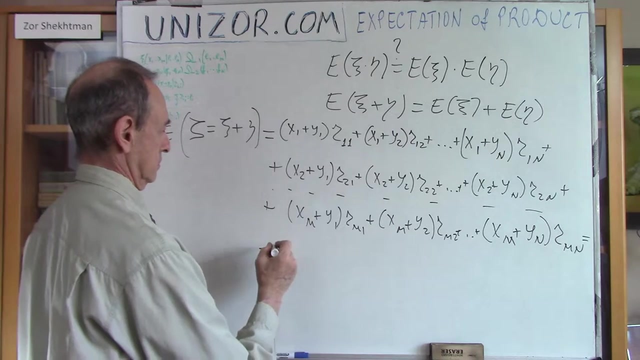 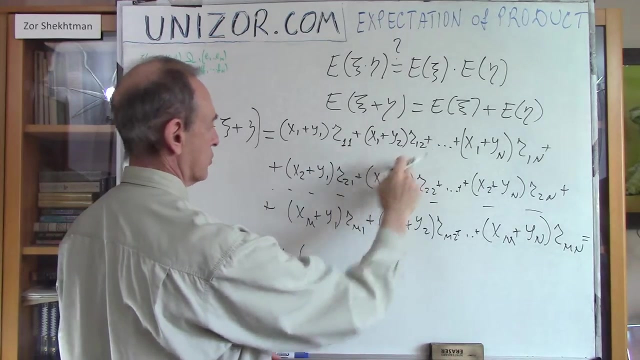 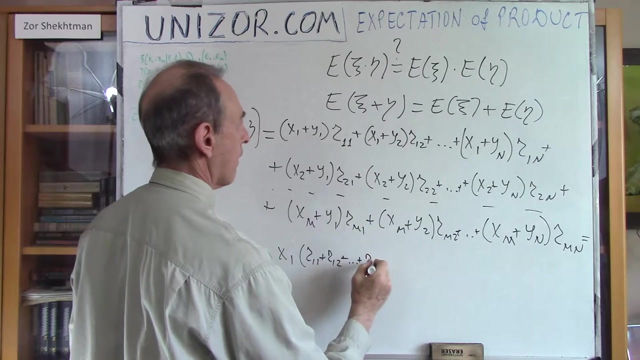 Now we will regroup it in this fashion: We will just open the parenthesis right And we will add together x1 times r11, r12 plus etc. plus r1n. And we will regroup it in this fashion: We will just open the parenthesis right. 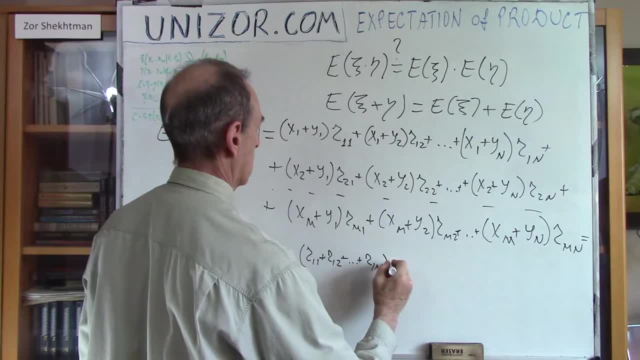 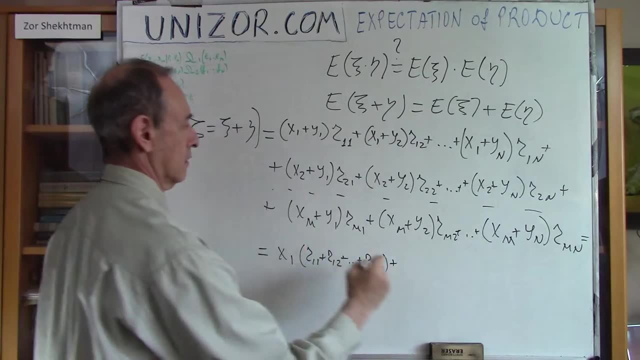 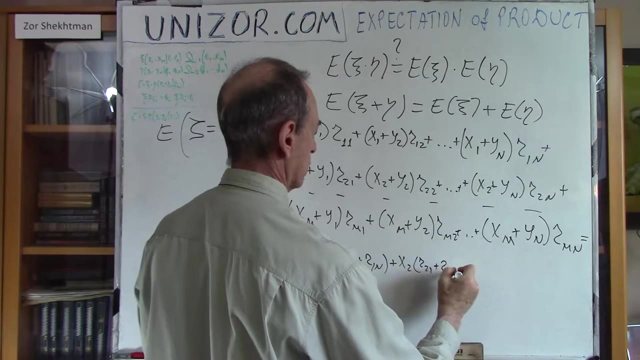 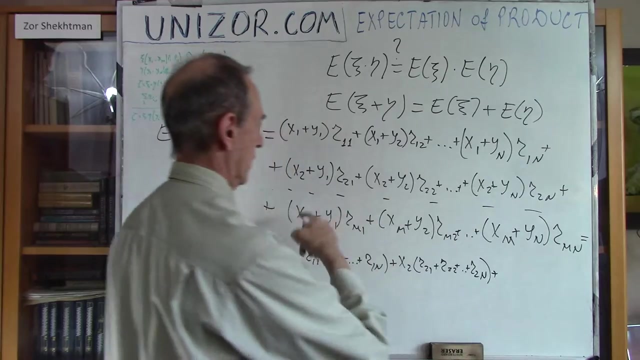 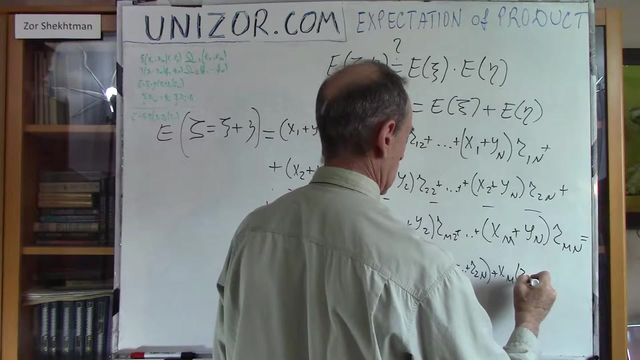 And we will regroup it in this fashion. So that's my probability. times r11, r12 plus, etc. plus xm. Okay, Then x2 from here. times r21, r22 plus r2n, etc. up to xm, M1, M2, Mn. 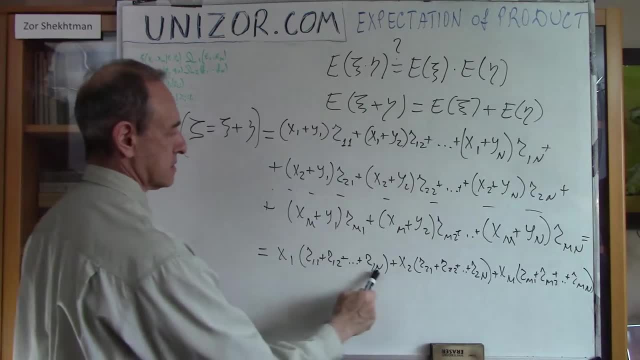 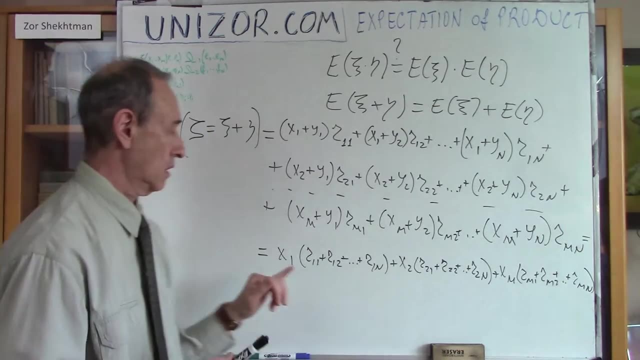 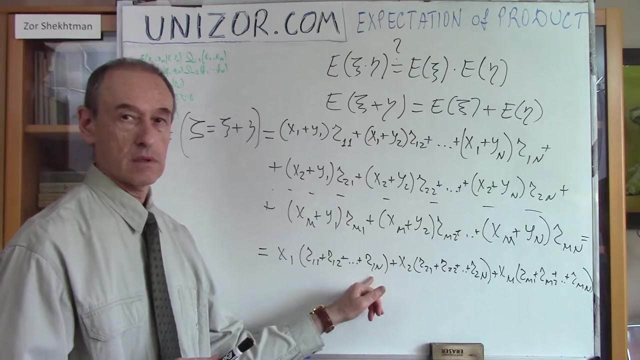 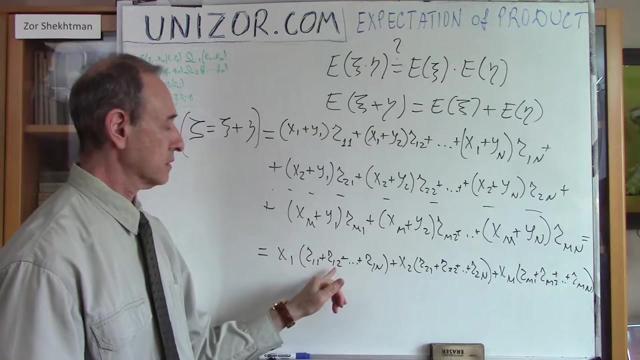 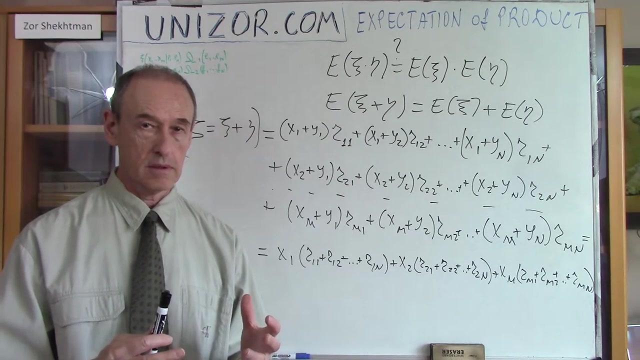 Now let's think about what is this sum? This summarizes the probabilities of X1 taking value 1 in all these cases and eta taking any basic value from Y1 to Y2 to Yn. So we are summarizing events when X1 is fixed. 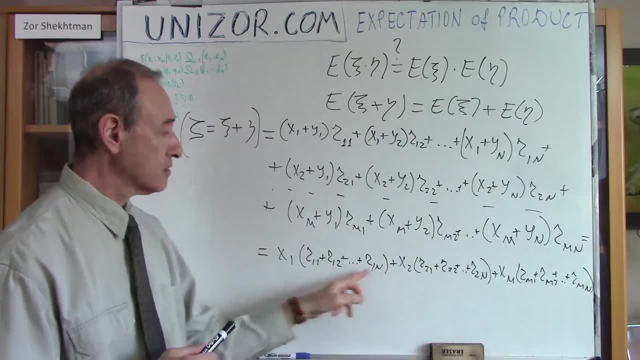 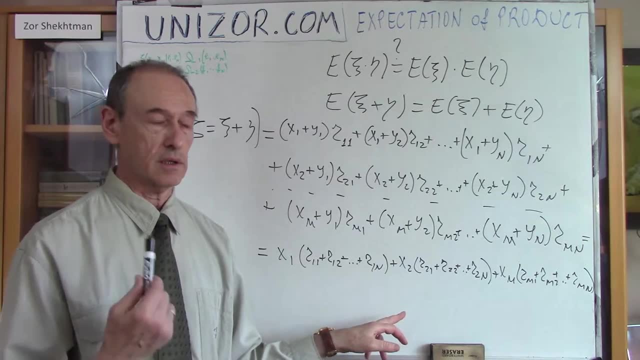 that's the value of xi, and the value of eta is not really fixed. it's basically any, because we are summarizing throughout all the values of eta, Which is basically from Y1 to Yn. Now what is this probability? 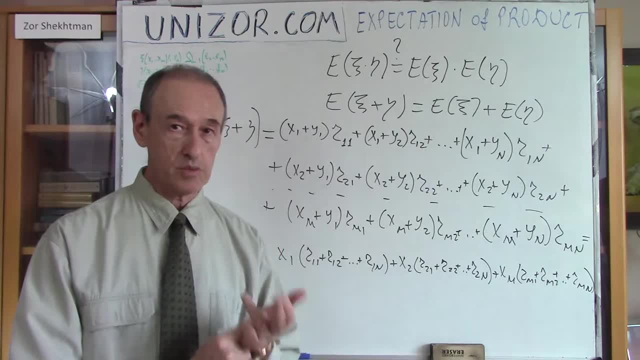 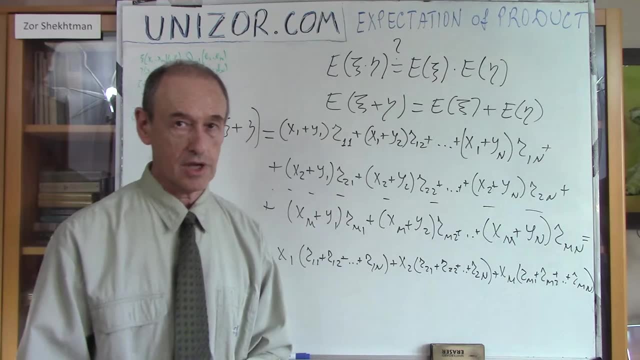 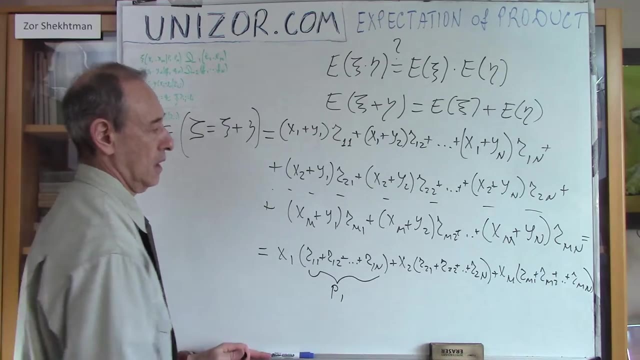 It's a probability of xi taking X1 and eta being any. We don't really care what value eta actually takes, right? Which means it's just the probability of X1 to be equal to P1.. And this is correspondingly P2.. 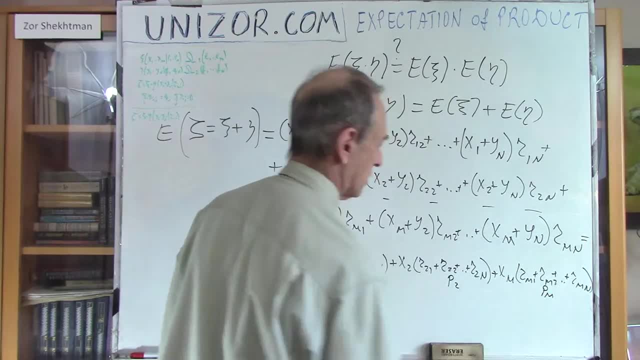 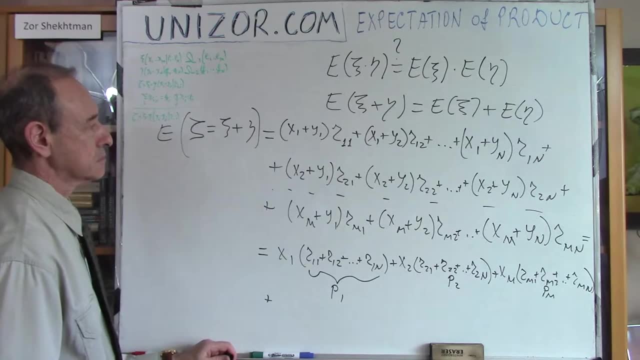 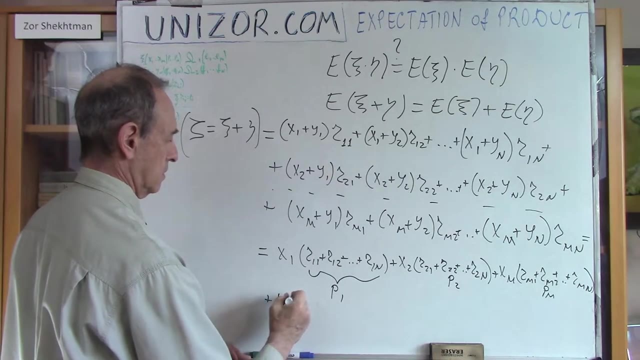 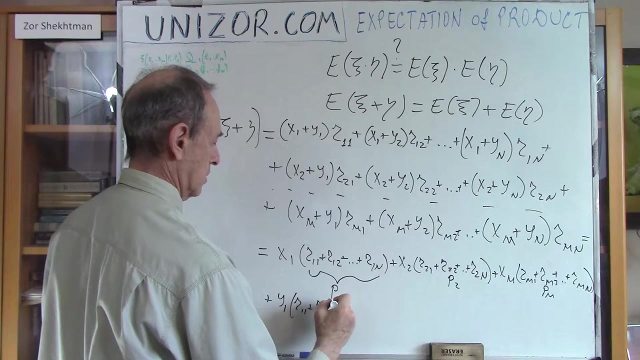 And this is correspondingly with P1.. P2, Pm: right, That's what it is Now. we'll continue. If we will continue, we will take Y, Y1 times R11 plus R12 plus, etc. plus R1n. 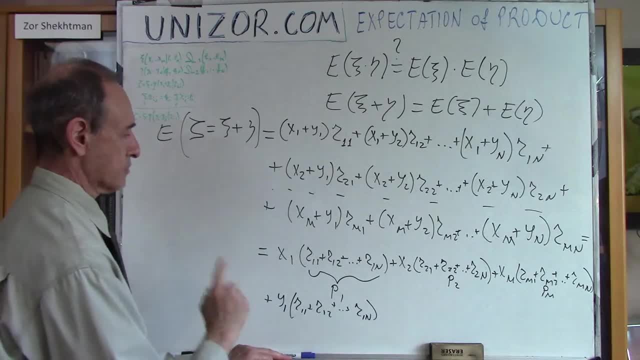 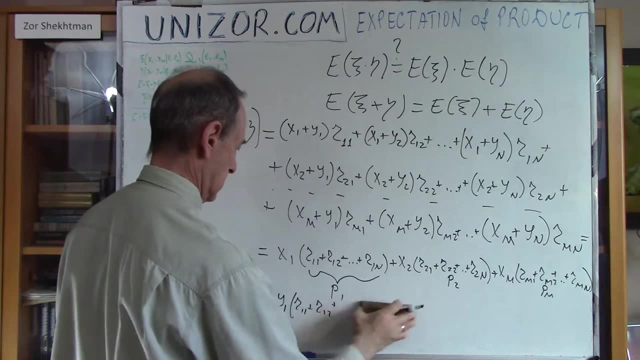 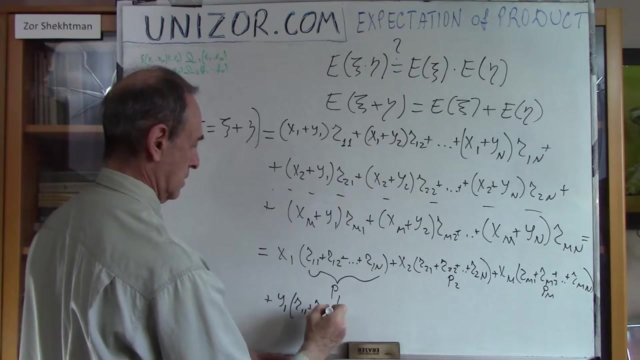 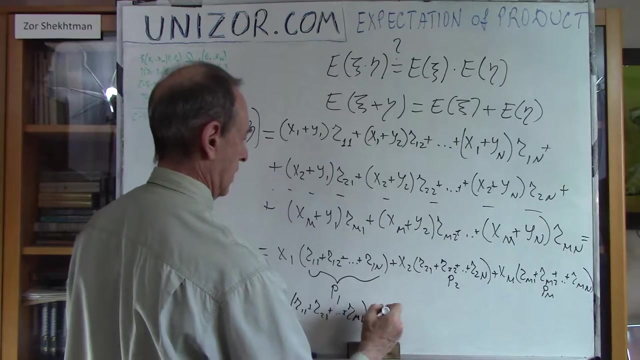 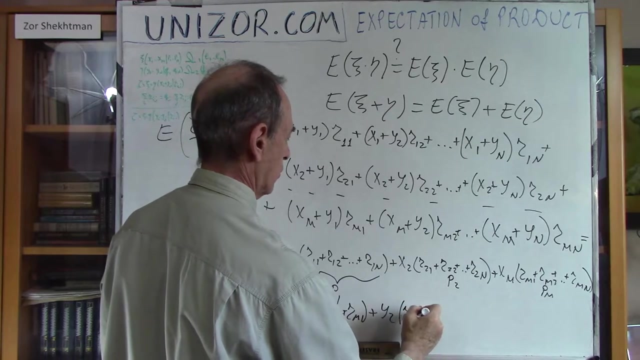 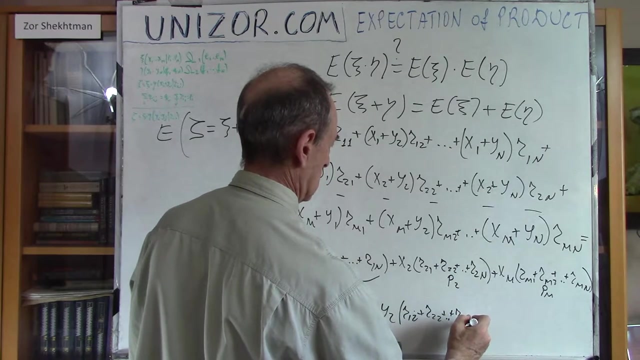 No, I'm sorry, with y we have to go down. yes, with y we have to go down, which means r11, r21, etc. plus rm1.. Now y2, y2, y2, y2, it's r12 plus r22, plus, etc. plus r2m2.. 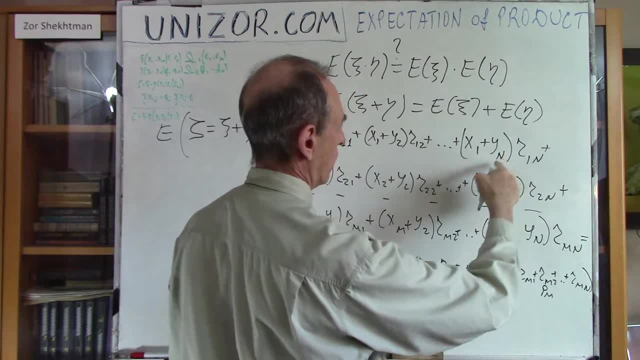 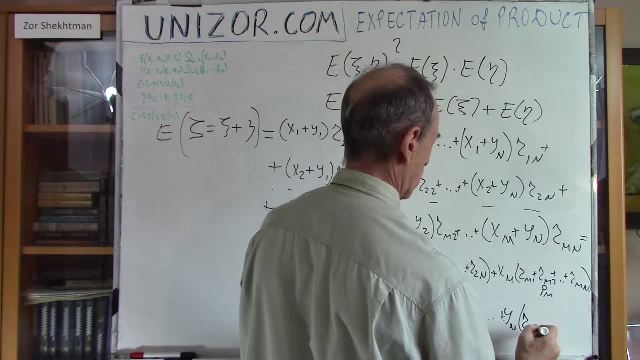 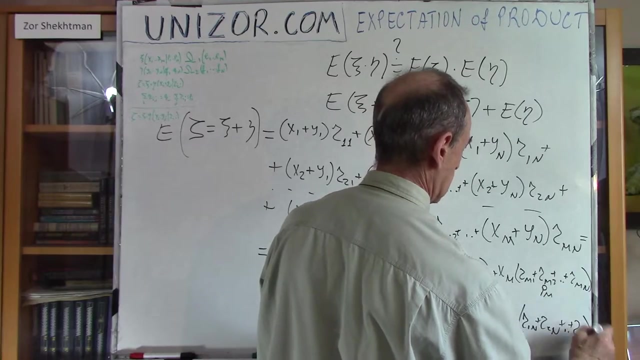 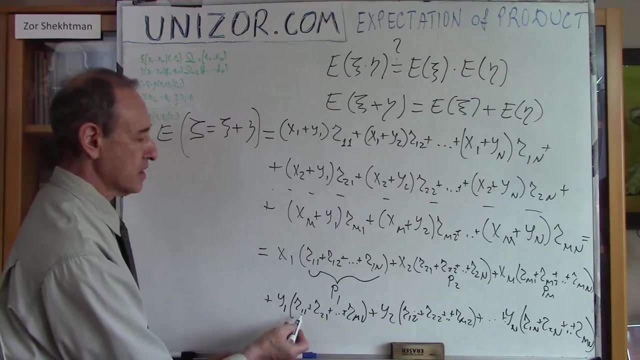 And finally yn, r1n plus r2n, plus etc, plus rmn. Now, what are these? Well, same thing. What is this probability? It's the probability of xi taking any value, either 1 or 2.. 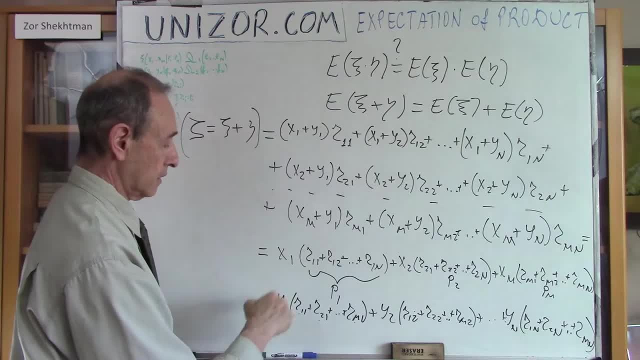 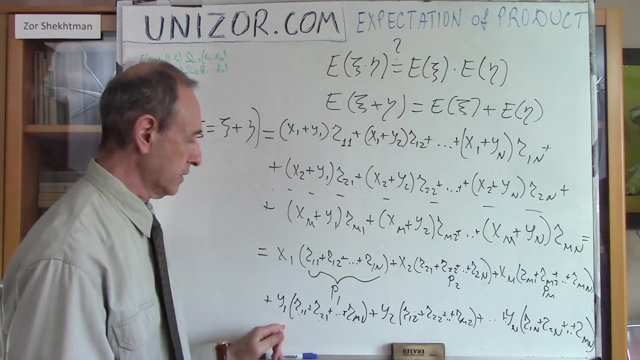 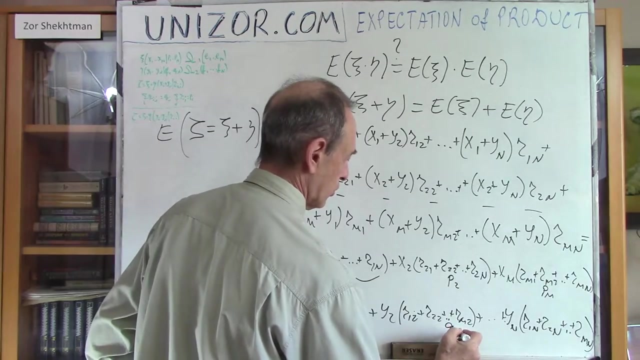 Or x1, or x2 or xm, while eta would be always equal to y1, which means what? So we care about only the value of eta, which is equal to y1, and any value of x, And that is q1.. This is q2.. And the last one is qn. 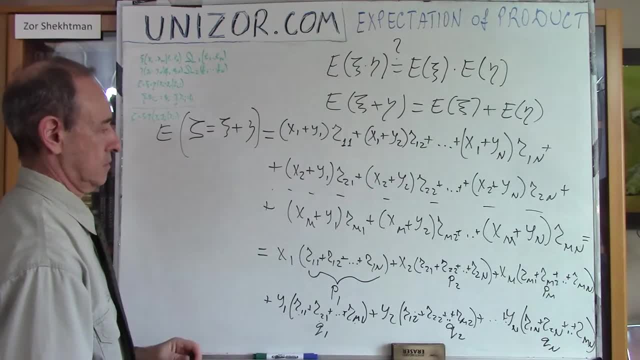 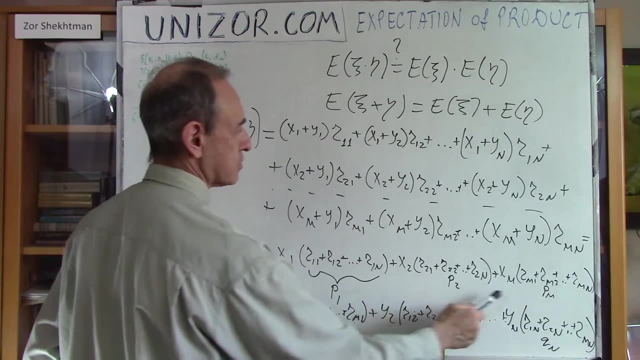 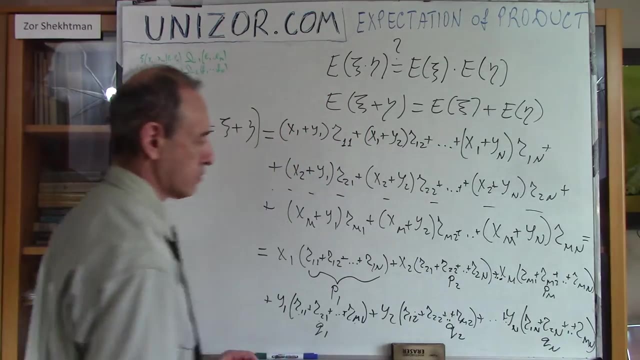 So So what do we have right now? We have this: x1 times p1, x2 times p2, and xm times, etc. times. this is etc. and the last one is xm times pm, which is expectation of this part. 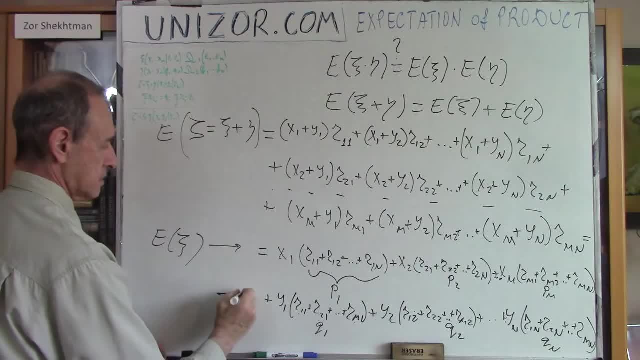 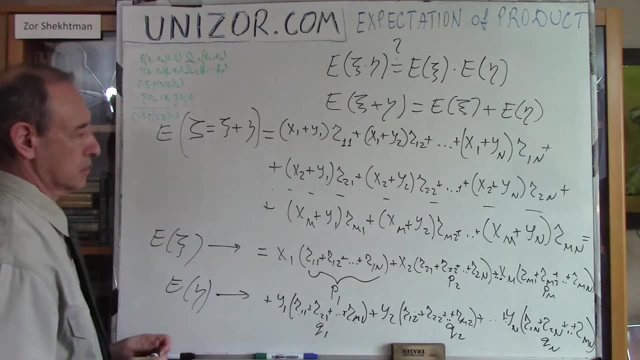 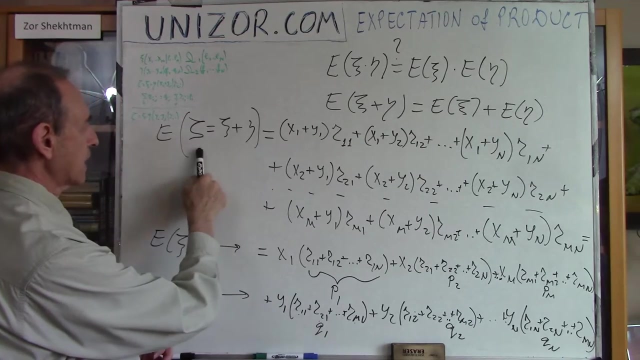 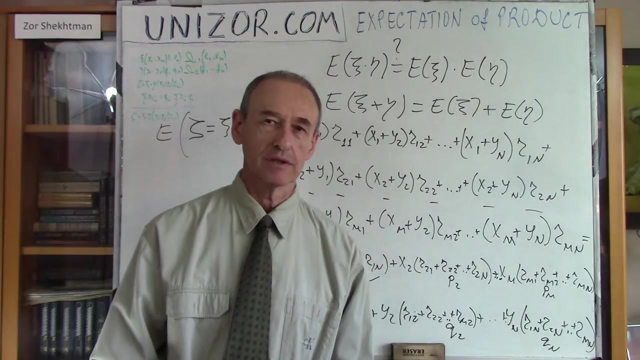 is expectation of xi and this one is expectation of eta. So, as we see, with sum of two random variables we always have that the expectation of their sum is equal to sum of their expectations. So why do I have some doubts about the product? 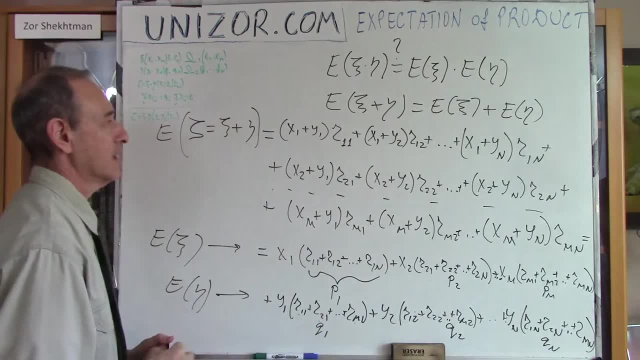 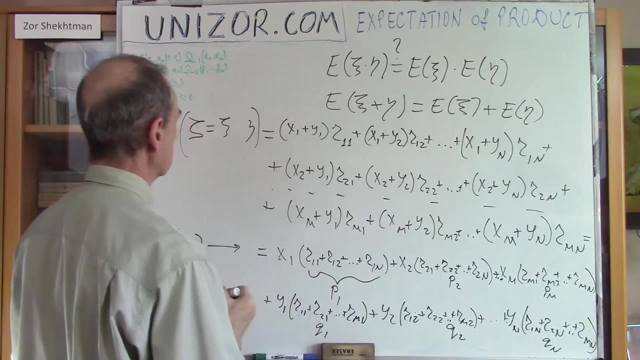 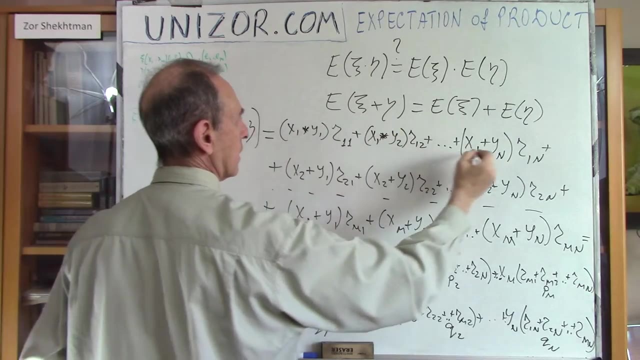 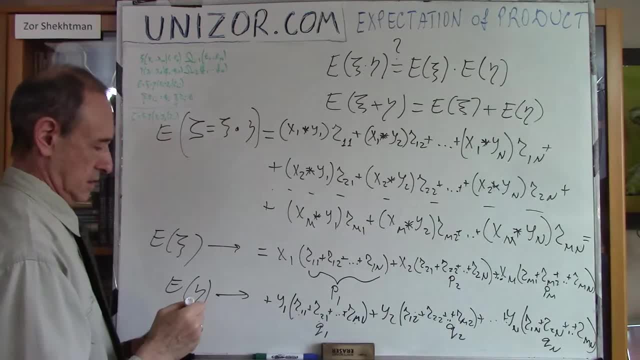 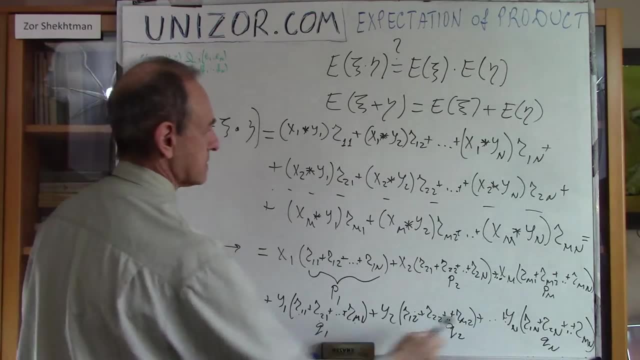 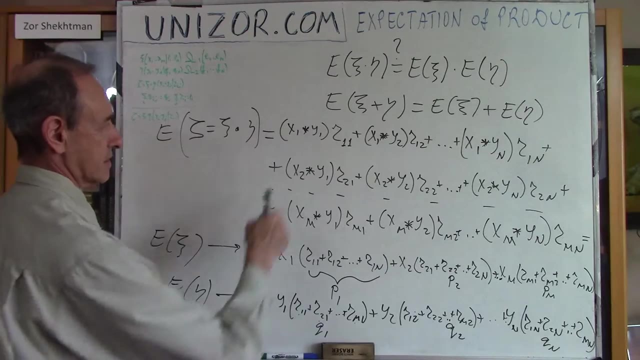 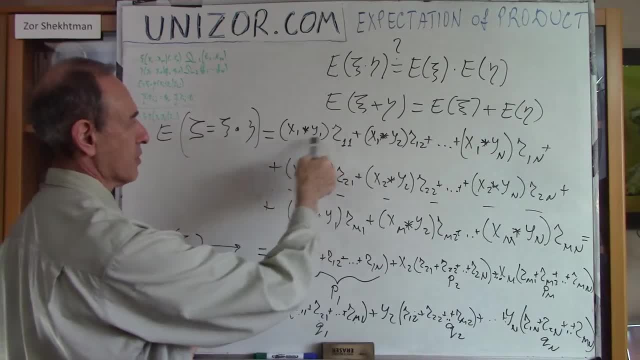 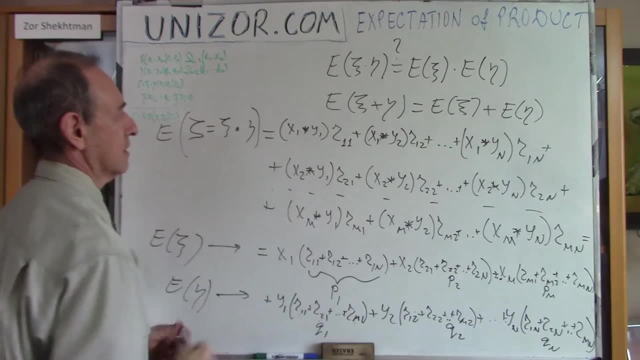 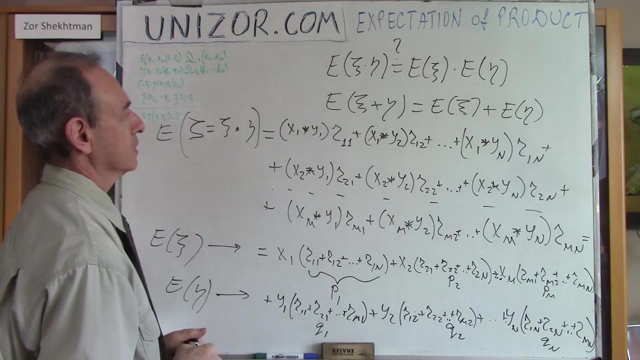 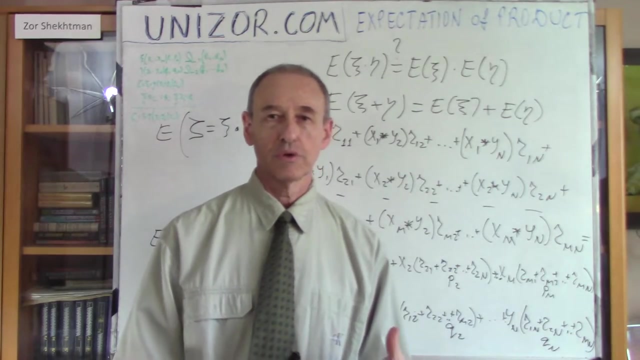 In the first place, when it was a plus. we have just summarized. basically, we opened the parenthesis and we have multiplied right With this. it's not that easy. So what can we do about this? Well, let me again jump up to the very end of this lecture. 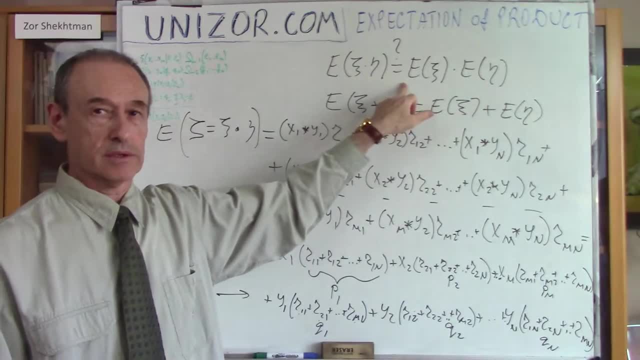 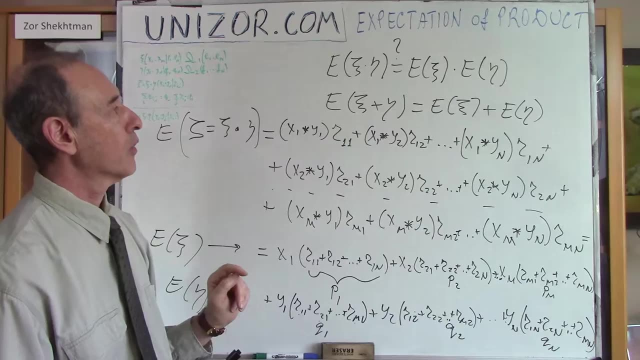 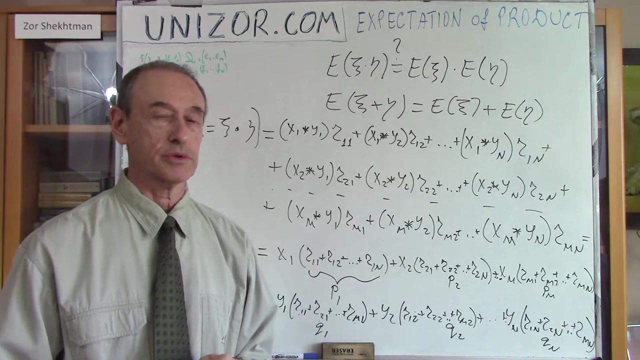 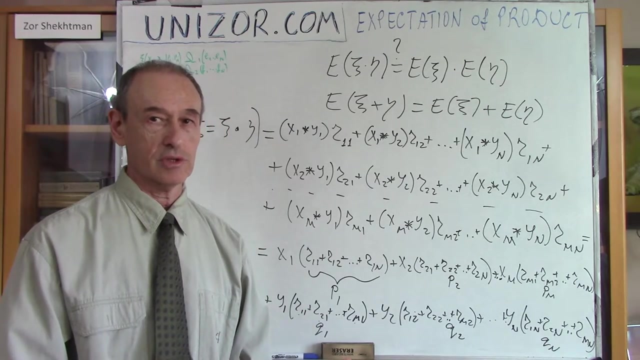 This formula is actually correct, but only in case when our variables xi and eta are independent. That's what's very, very important. And to go further, I would like actually to remind you what independence actually means. Again, you can always refer to the lecture about independence. 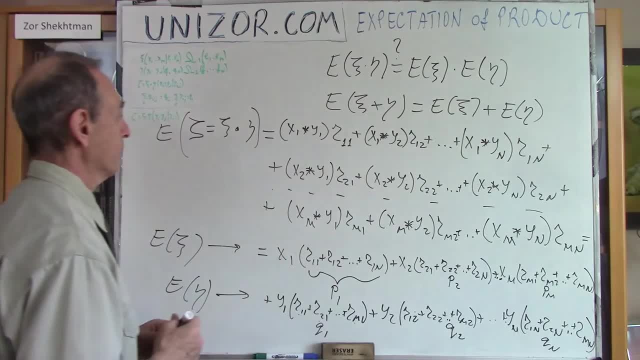 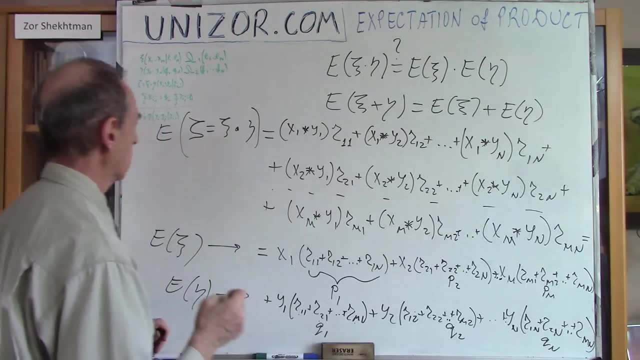 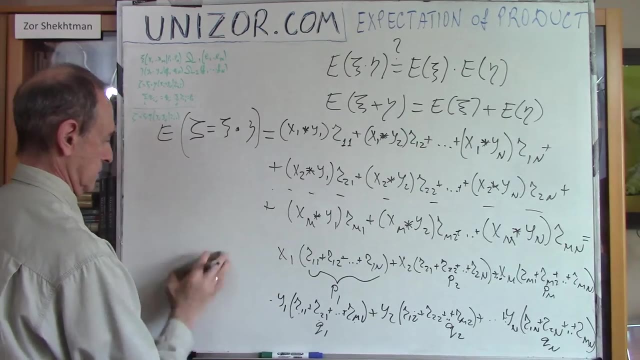 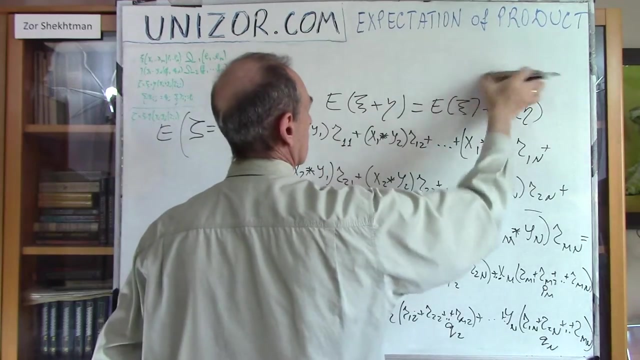 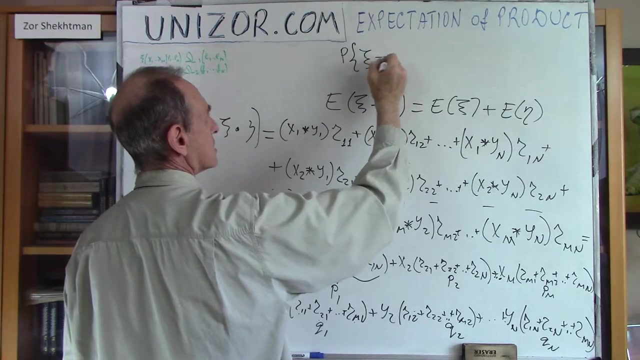 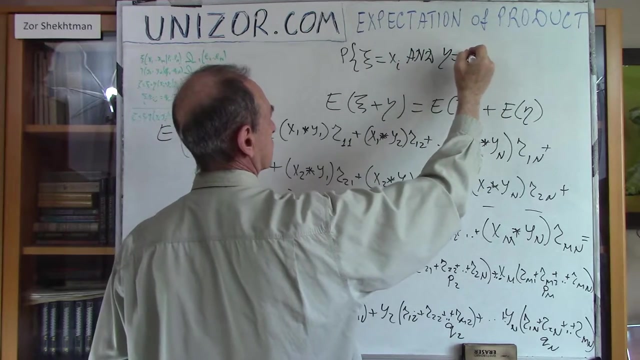 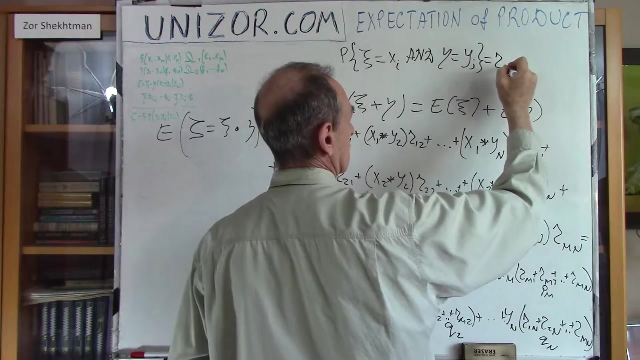 Random variables, But in particular, independence means that the probability, The probability- Actually, I don't need this anymore, We know what we have to prove. Let's say, probability of xi is equal to xi and eta is equal to yj, which I have actually suggested to write it as this one. 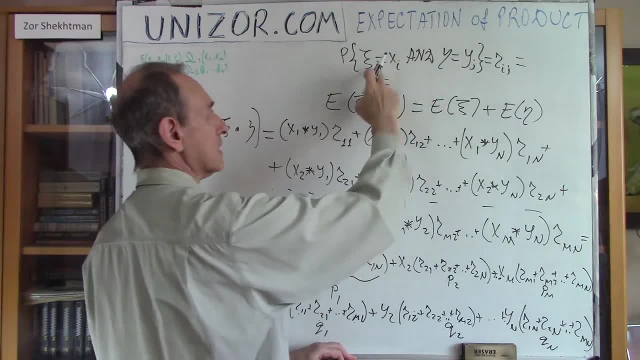 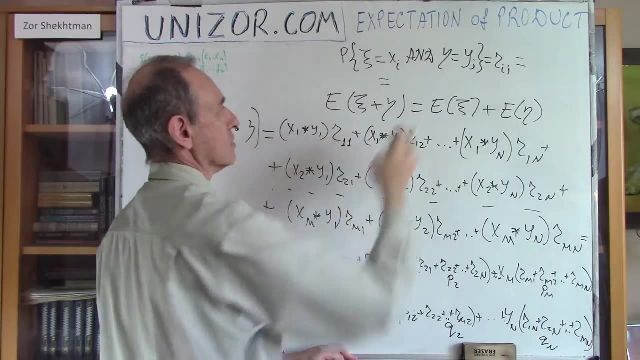 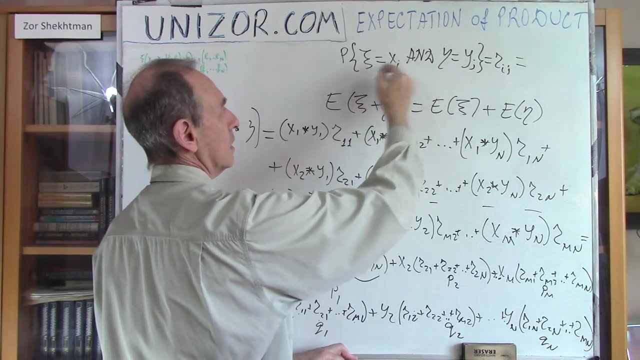 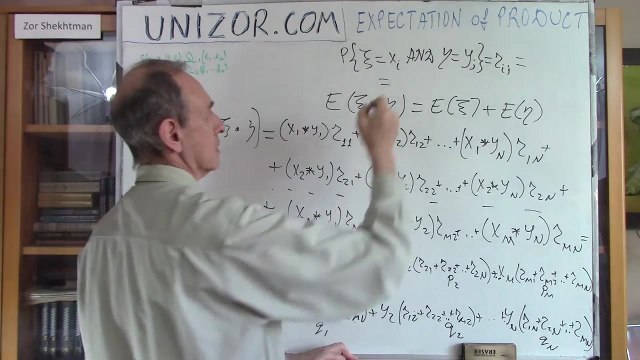 Equals to: It's the probability of the combined events. Now, if xi and eta take these values, xi and yj, independently, then we know that the probability of intersection of two events is actually equal to the product of their probability. 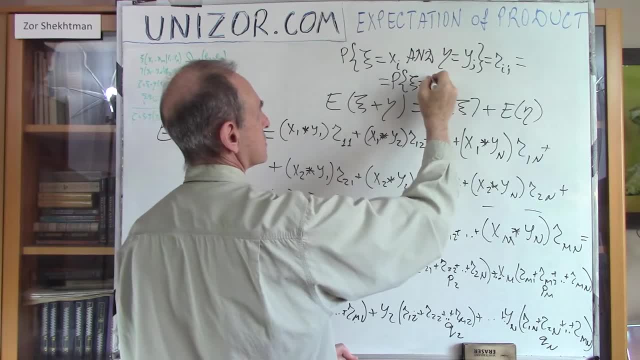 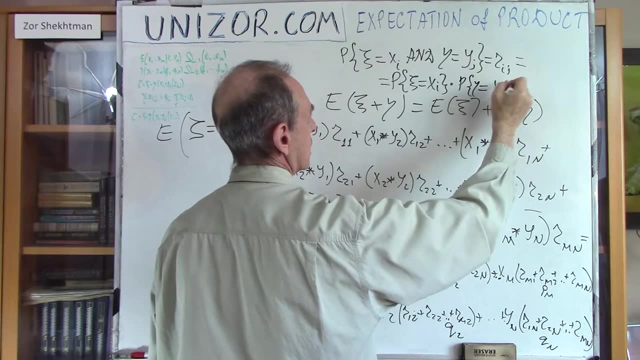 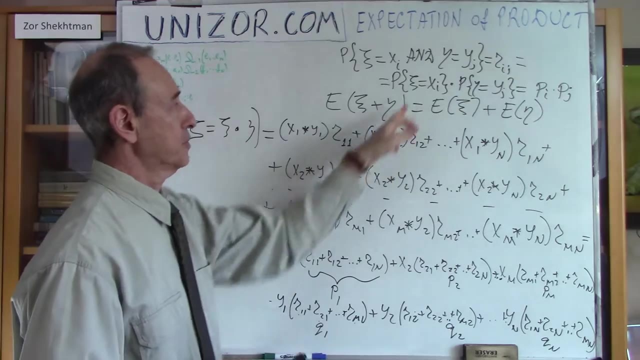 So it's the probability of xi equals to xi times probability of eta equals to yj, which is pi times pj. Right pi is the probability of xi to be equal to xy and- Oh, I'm sorry, it's qj. 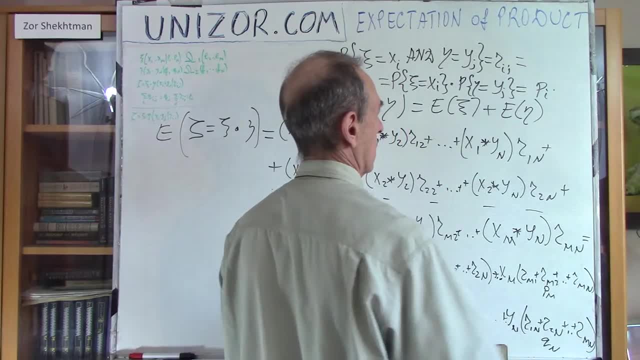 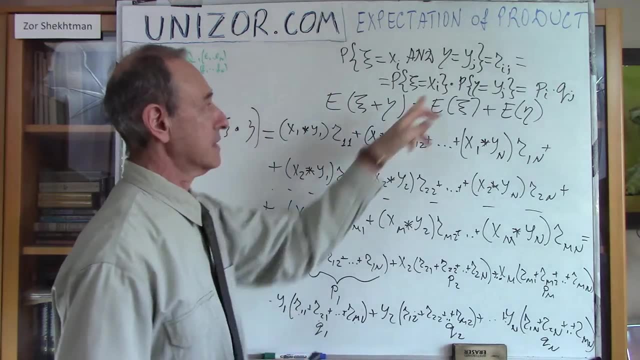 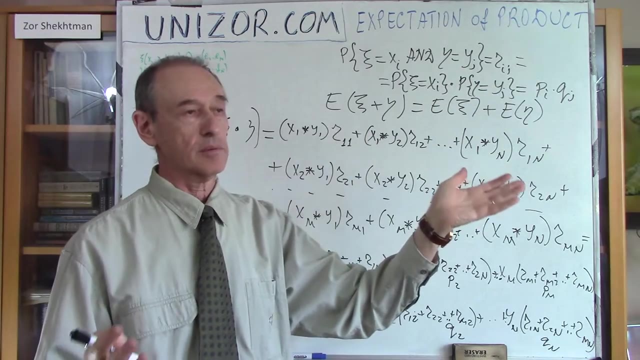 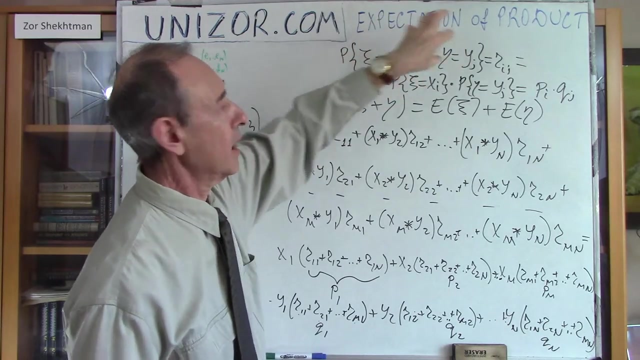 It's q. So that is a very, very important property of independent variables. It's basically a property of independent events, This being one event and this being two events, This being one event and this being another event, And combined events if events are independent. 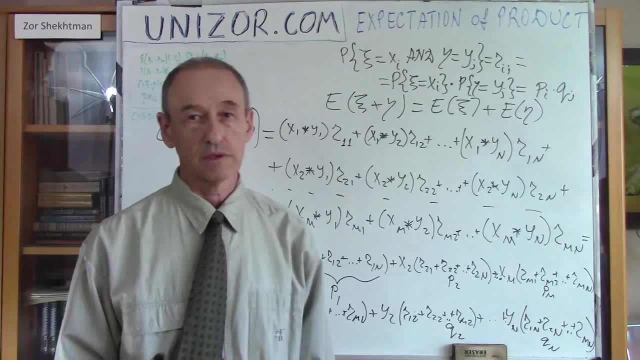 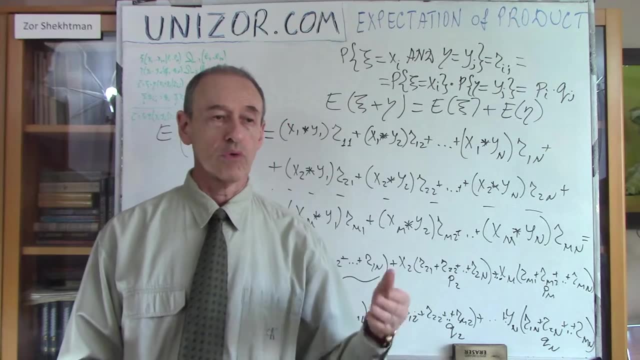 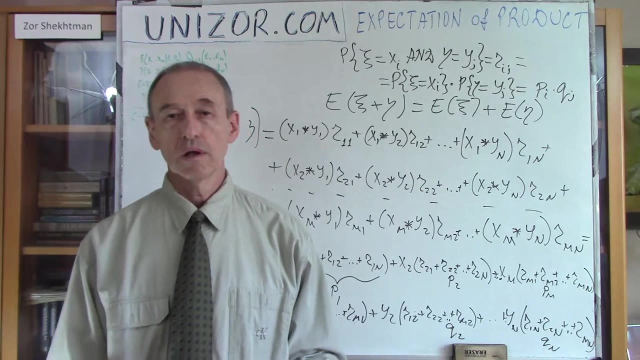 the probability of the combination is equal to the product of two probabilities. It's like the probability of one die to fall on number two and another to fall on, let's say, number four. Well, it means the combination of two dies. 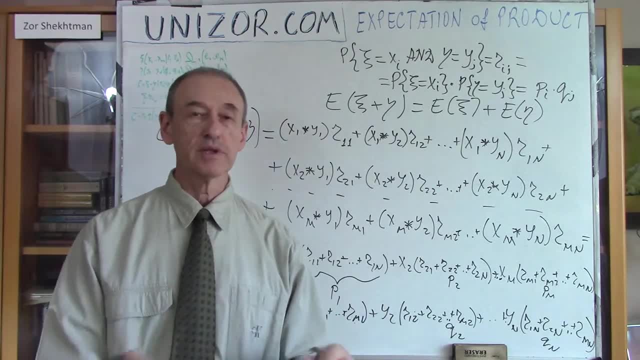 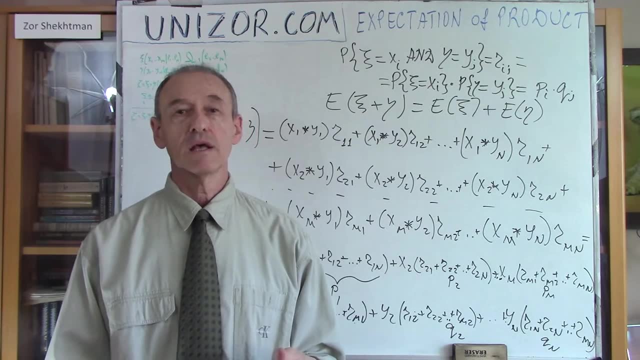 is two four, And the probability of this is one thirty-six. obviously right, Because there are thirty-six pairs, But at the same time, this one thirty-six is equal to one six times one six, which is probability of the first die to be. 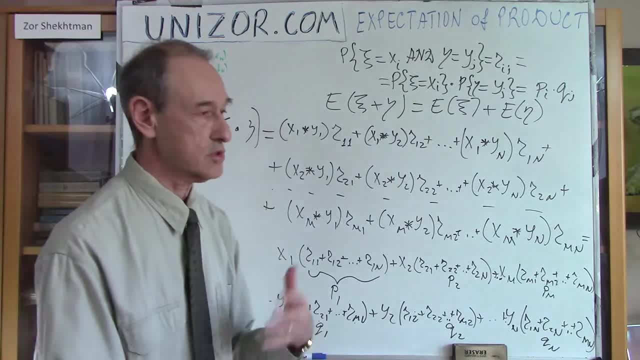 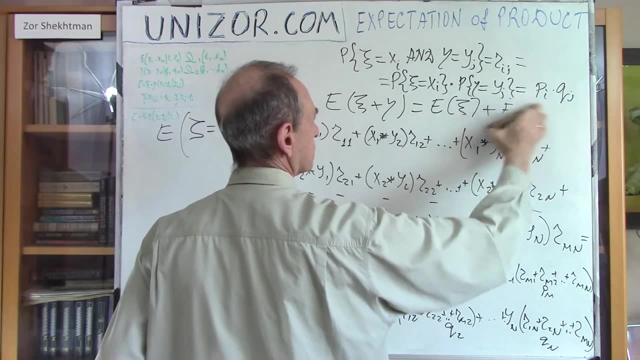 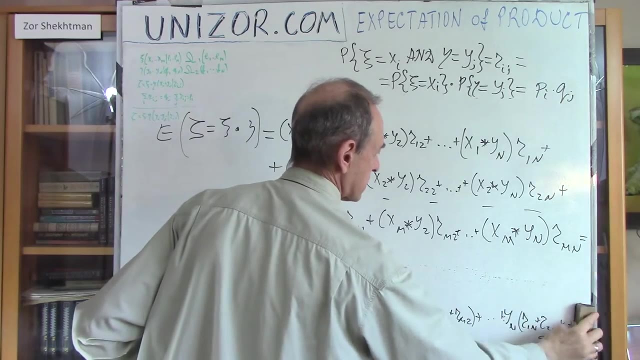 to fall on the two and the second to fall on the four. So it's always like this for independent events, And that's what we are going to use in this particular case. So let's forget about this. This is absolutely not working in case of a product of random variables. 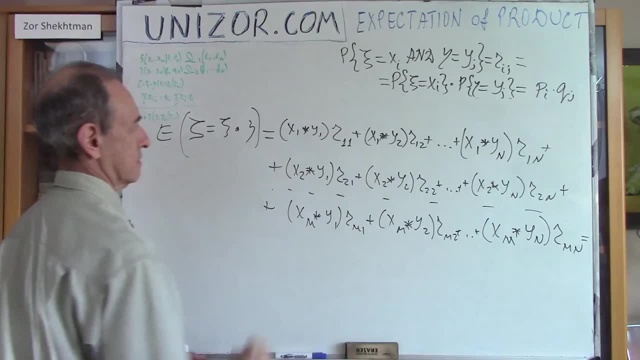 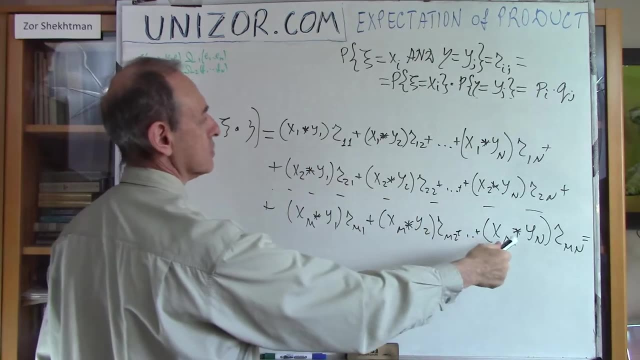 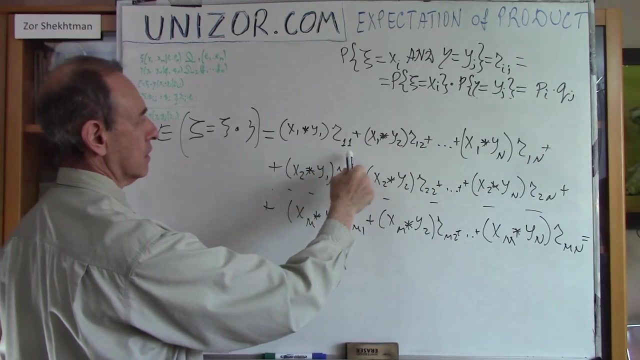 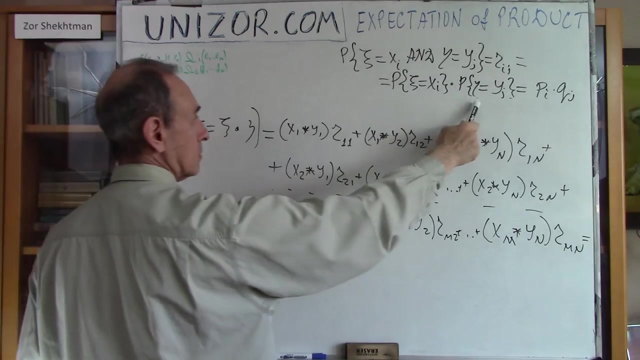 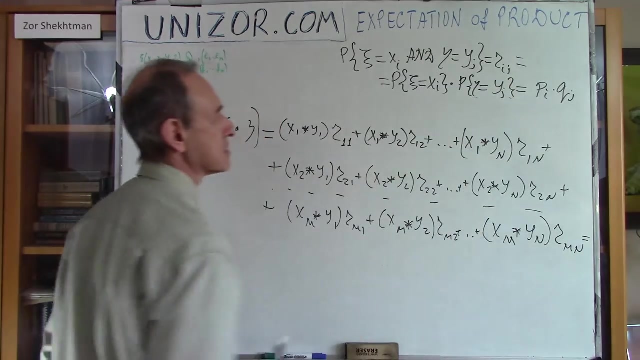 But we do have this: All the different x, i and y j are different values which our product can take, And r i j is the corresponding probability of this. But as we know here every r i- j is equal to p i times q j. 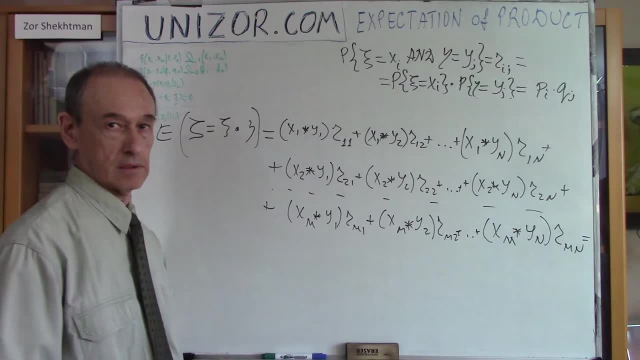 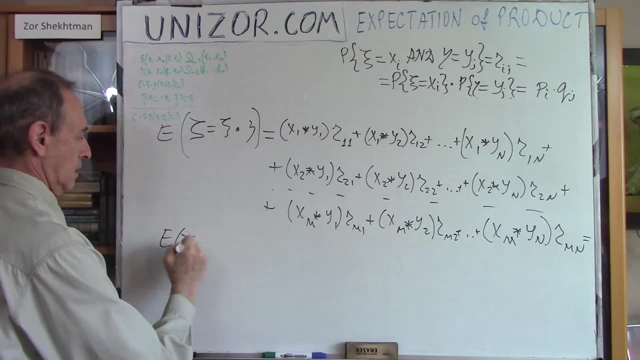 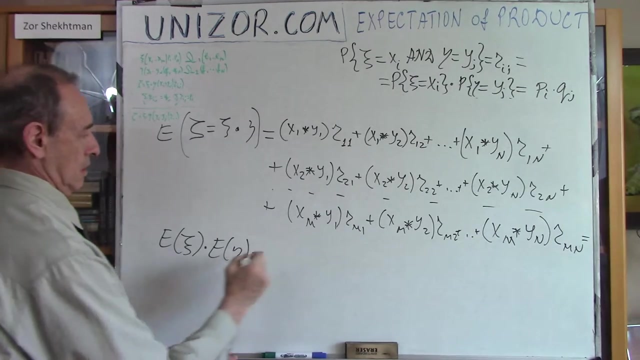 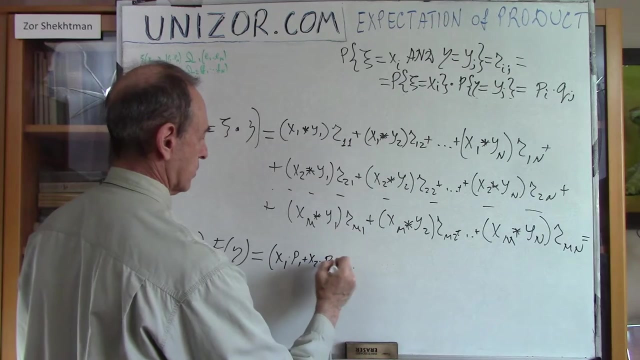 for independent xi and eta independent random variables. So let's consider what happens if I will do this. Times is equal to x one times p one, plus x two times p two, et cetera. plus x m times p m. 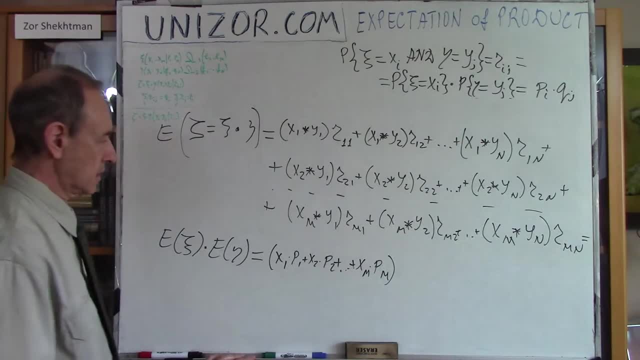 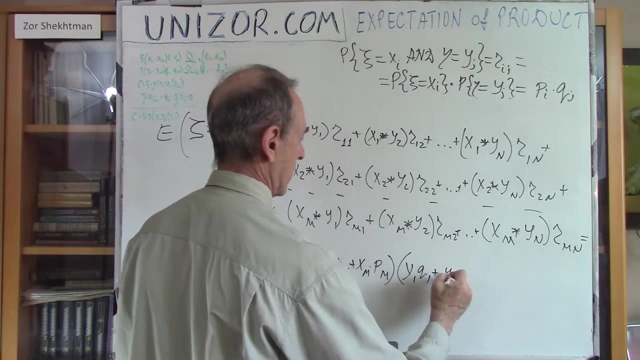 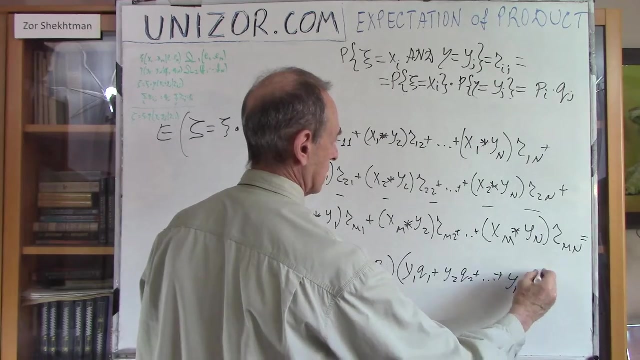 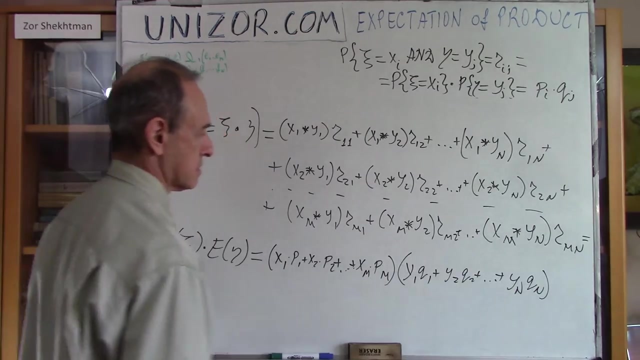 That's the expectation, mathematical expectation of xi times y one, q one plus y two, q two plus et cetera, plus y, n, q, n. Right Now, what if I will open the parenthesis and multiply this times this? Well, I will have. 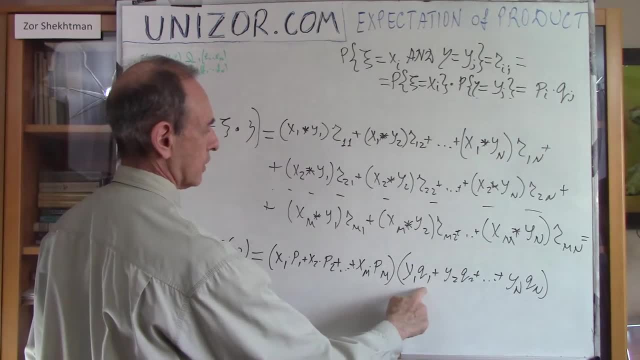 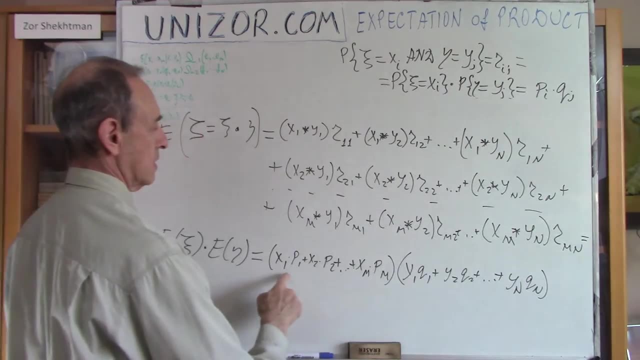 x one p one times y one, q one right Plus x one p one times y two, q two plus, et cetera. Then I will take x two and multiply by each of them, et cetera, et cetera. 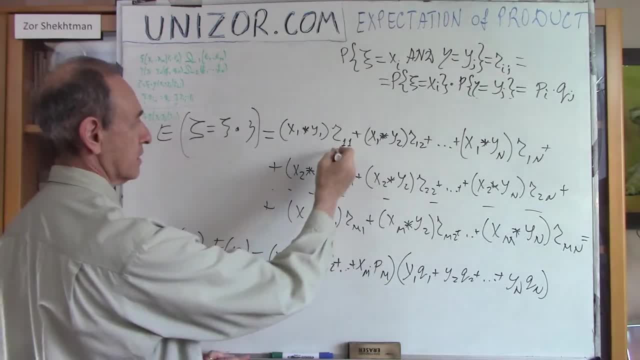 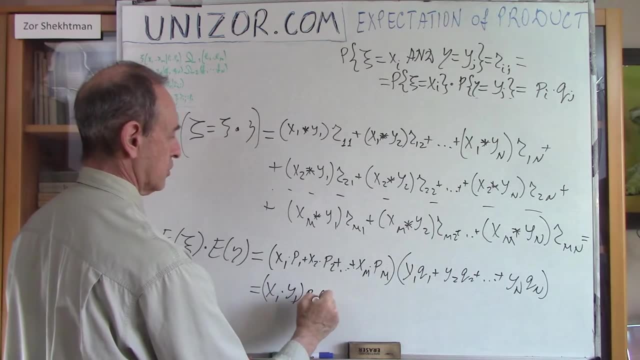 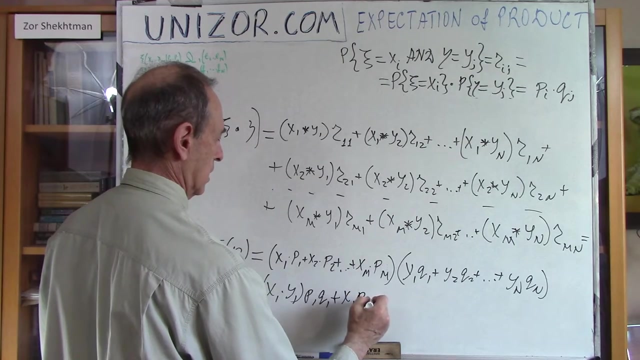 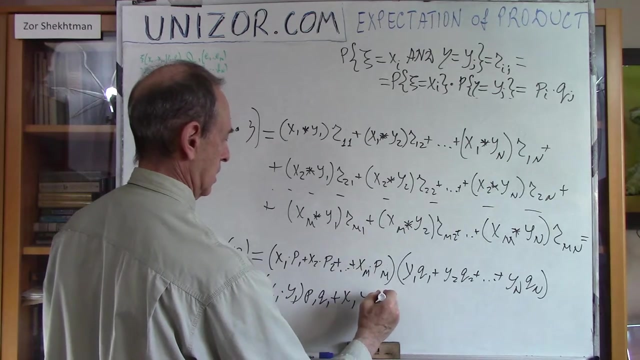 So what will I get? I will basically get this, but instead of r I will have x one times y one, p one, q one, right This times this, Plus x, one, p one, x one, y two, p, one, q two, et cetera. 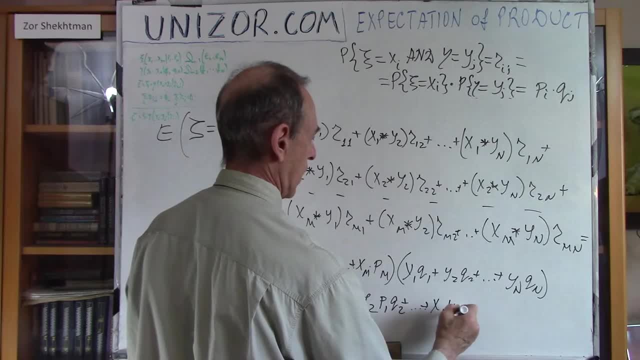 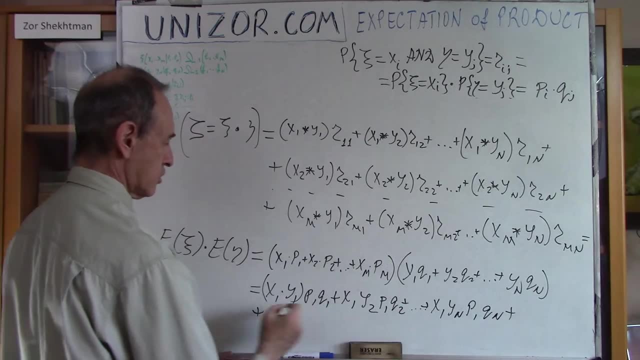 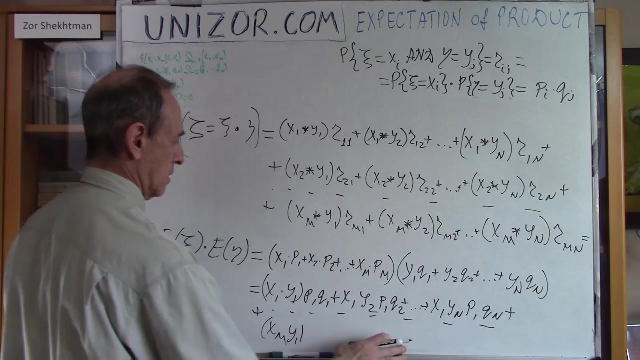 And the last one would be x one, y n, p one, q n plus. Then I will do the same thing with x two where x three, et cetera, and I will finish with x m times y one times p m. 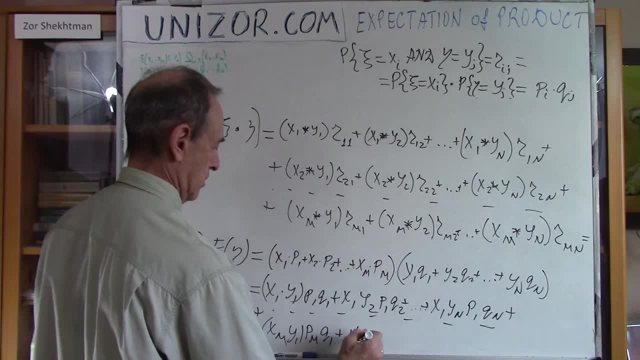 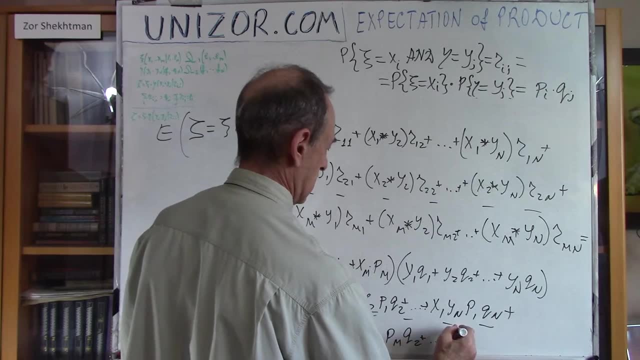 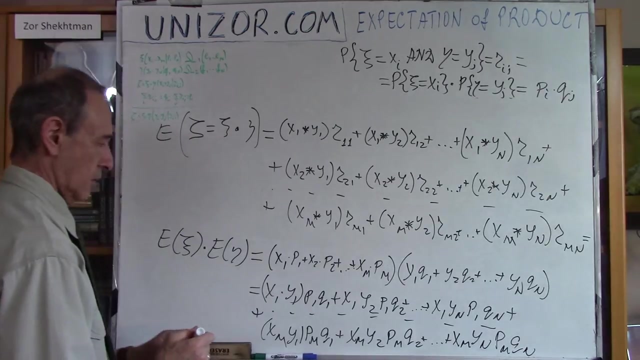 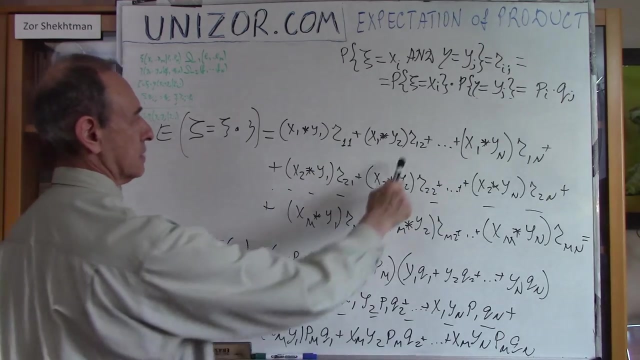 q one plus x m y two, p m q two plus et cetera, plus x m y n, p m q n. So it's exactly the same as this one, except instead of r one one I have p one q one. 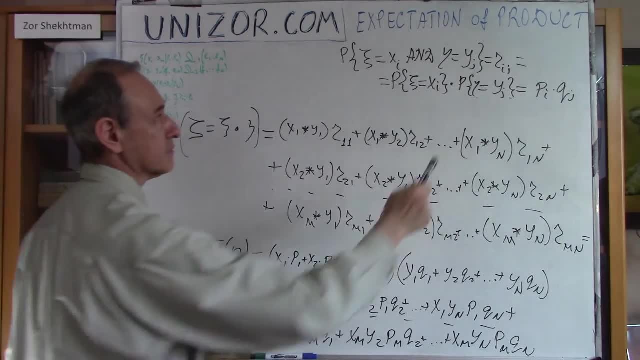 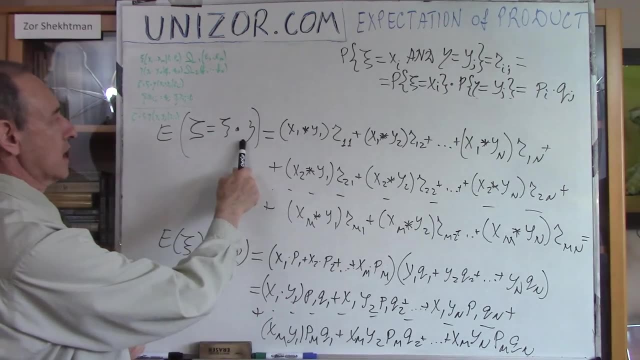 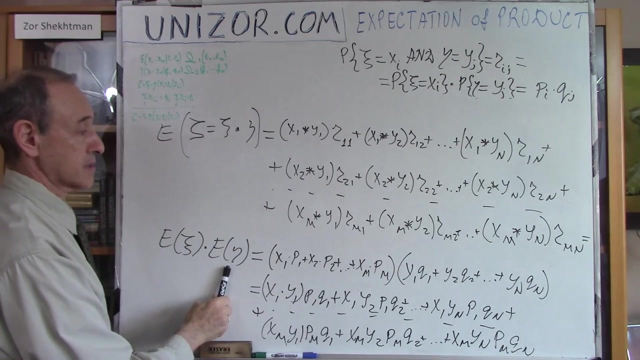 Instead of r one, two, I have p one, q two, But for independent variables they are equal to each other. That's why I can say that this mathematical expectation of the product of two random variables is equal to product of their mathematical expectation in case they are independent. 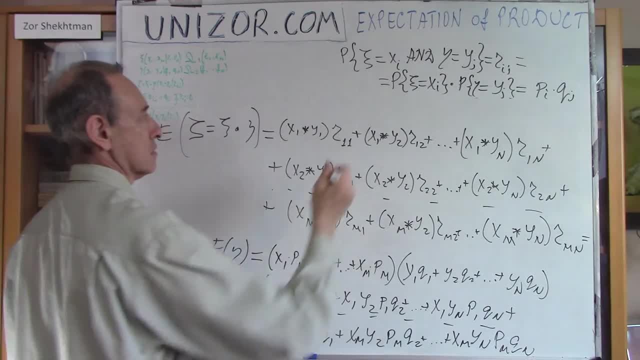 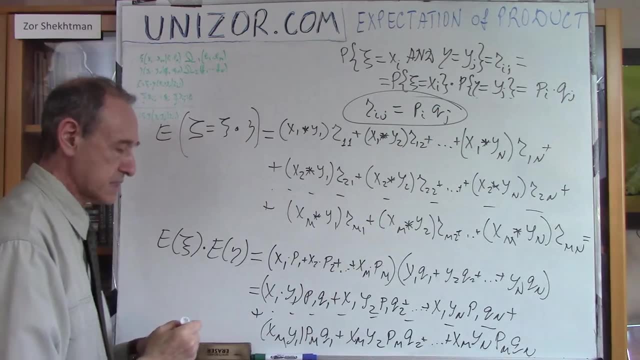 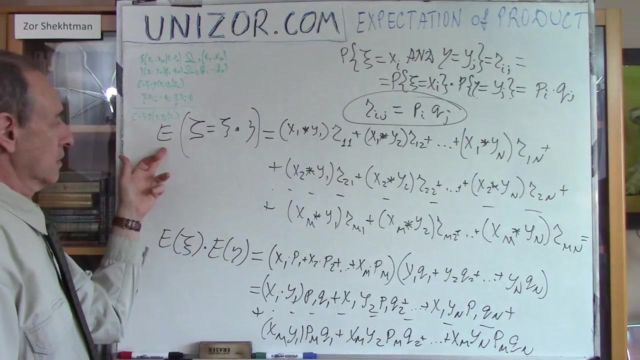 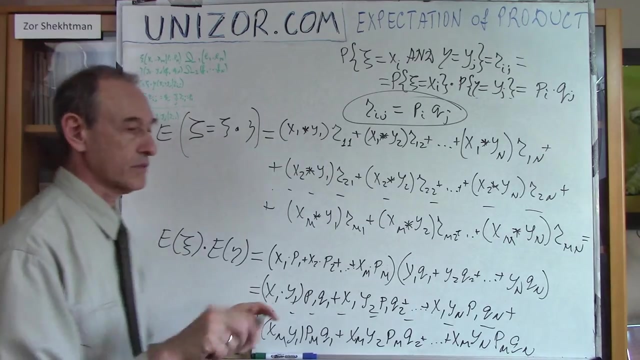 and this relationship is true. So if this is true- this is the key- then both expressions are basically the same: Expression for mathematical expectation of the product of two random variables and the product of their mathematical expectations. So this is the key. 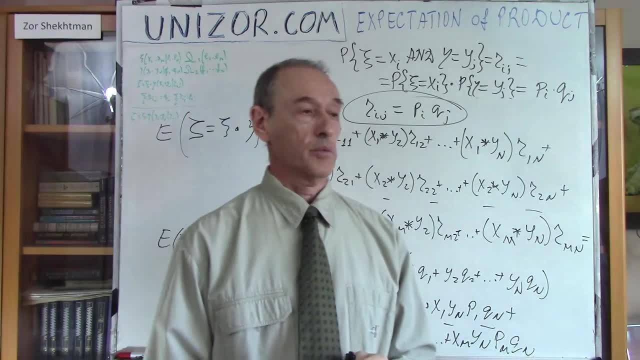 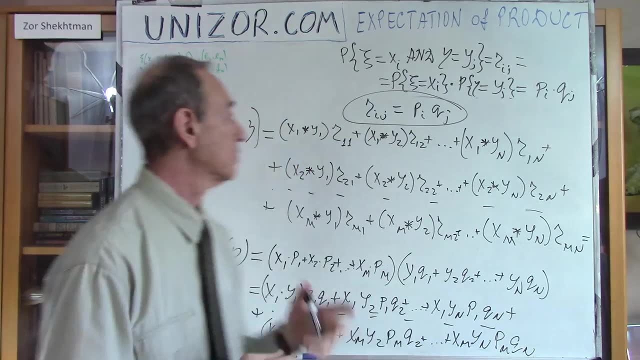 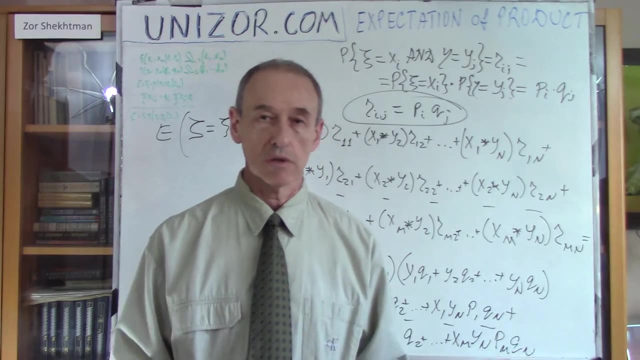 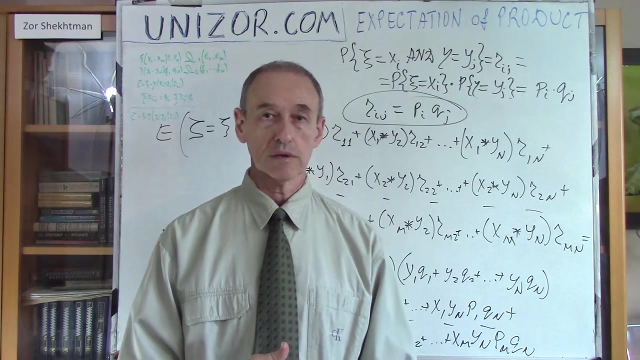 Independence. Well, so you see, there is a significant difference between sum and the product of two random variables. In case of a sum, we have this unconditionally- that expectation of the sum is equal to sum of expectations In case of a product of two random variables.